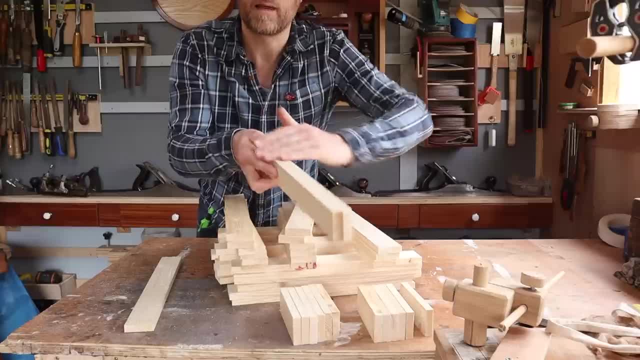 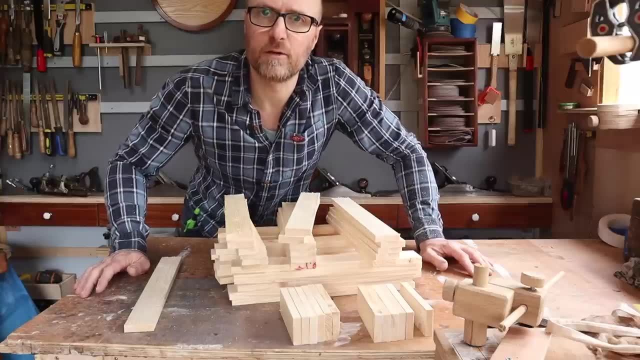 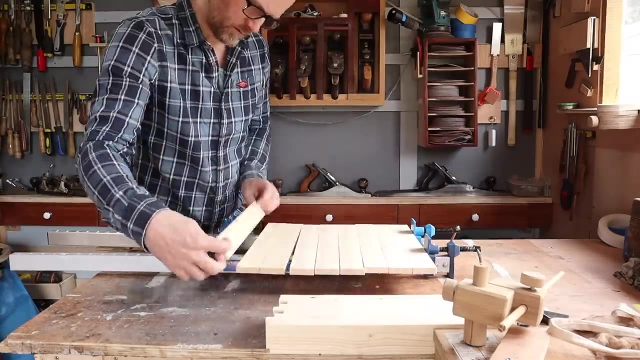 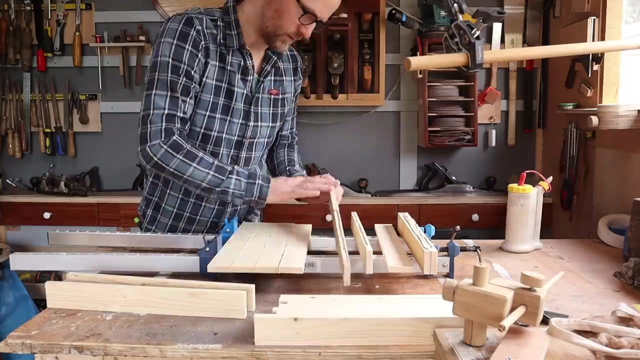 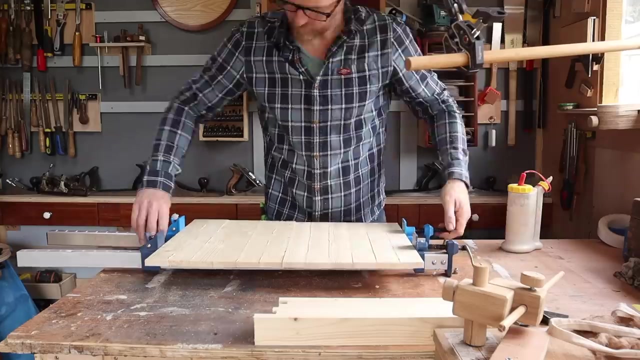 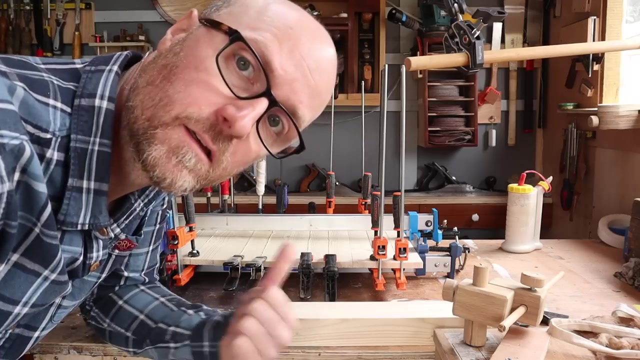 joints is: open it like a book, clamp it together, plane it, close it again and you'll get a really tight edge. So let's get it glued up. That was frantic, but it'll get the job done. These have come out of clamps. now. If you've got a thicknesser, send them on through. You can do it. 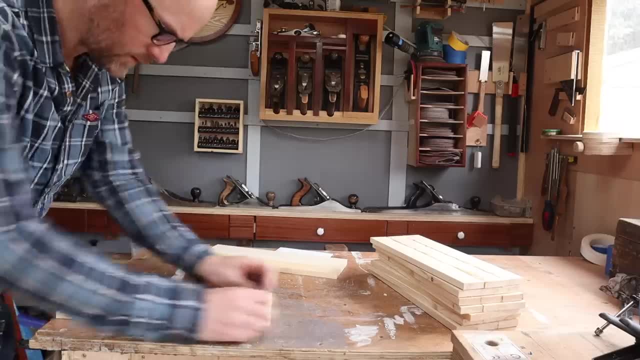 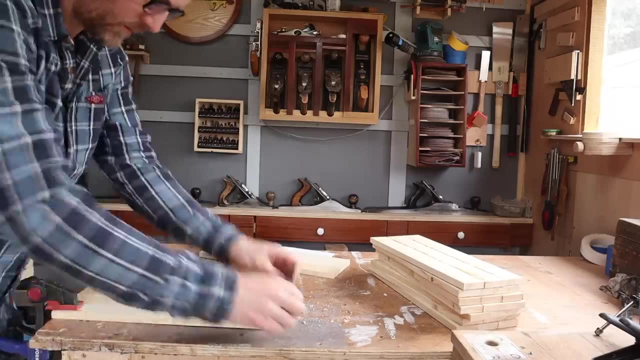 with a sander. I'm just going to quickly plane them all down, mainly because I quite like planing pine. Don't take too much off, because they're already quite thin, and then we're going to cut the sides and get it all glued together. 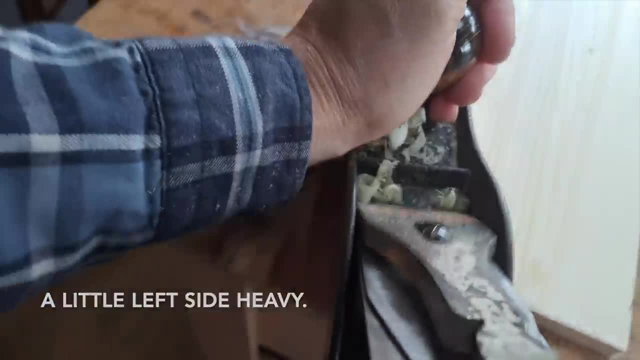 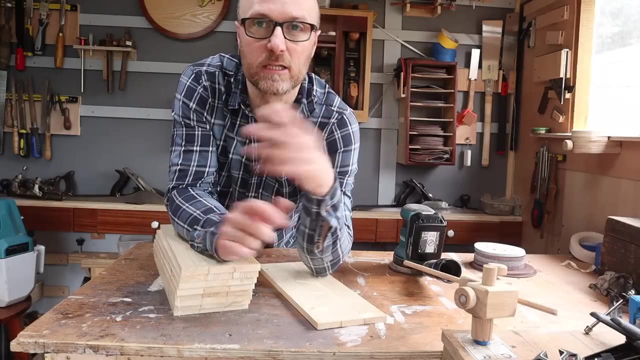 I confess I did not try and get a finish with the plane on these. I just used it to level them out. it wasn't sharp enough really to get a crisp finish, so now I'm going to sand them. All you're doing is getting to the insides because you can't get to them later. 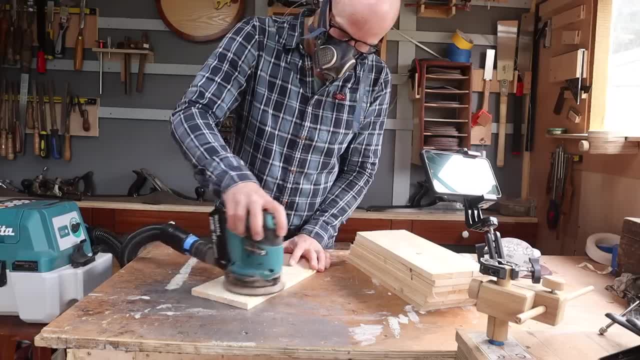 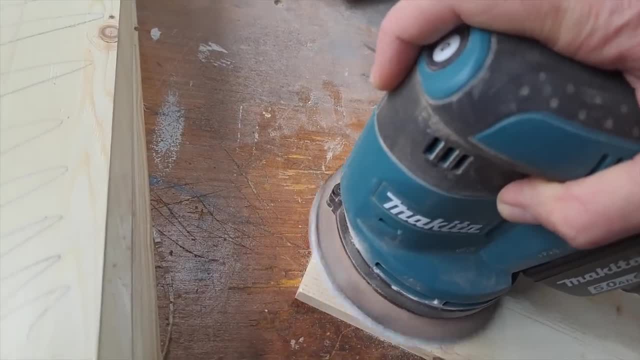 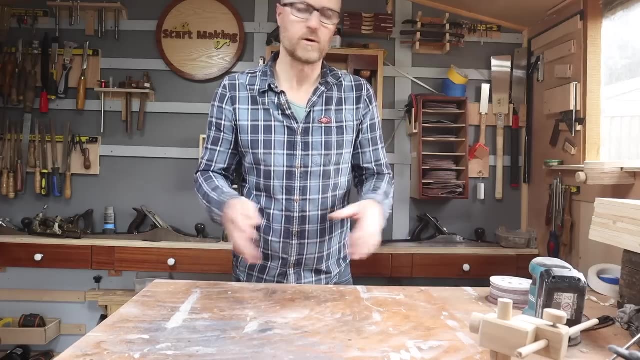 and then we're going to pick what we're going to use for each piece. The next bit we're going to build is the surround of the box. To save a bit of cutting later, I've just cut these to be about 4 to 5mm. 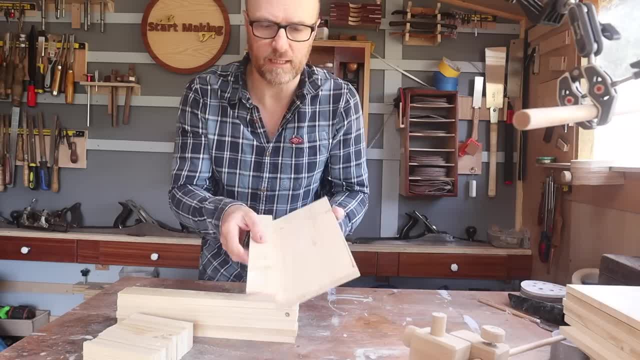 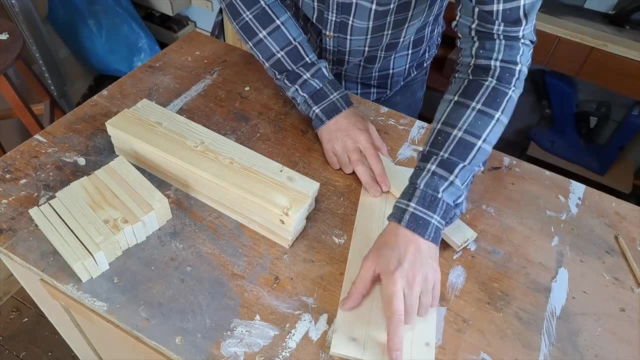 shorter than the ones we used for the tops and the base. The reason for that is it just means that the tops, if you haven't got the ends perfectly aligned, that means we've got some trimming space and it's going to be as close to the length of the finish box as 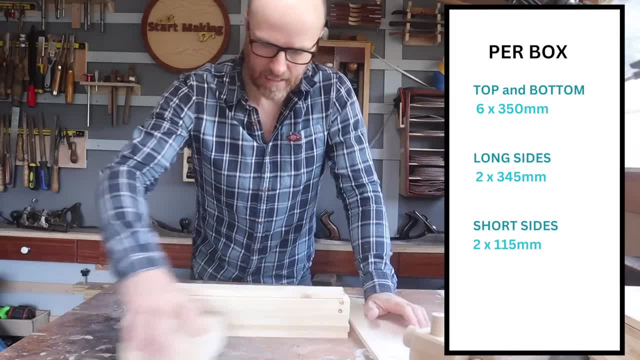 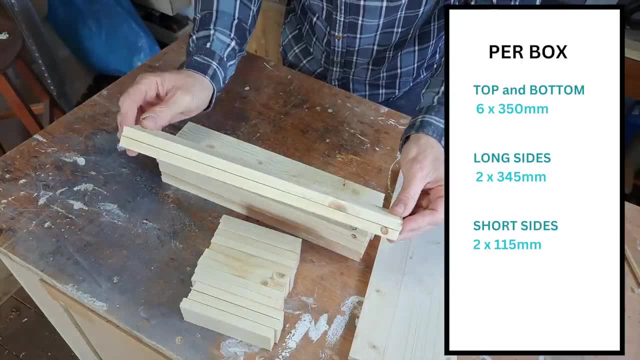 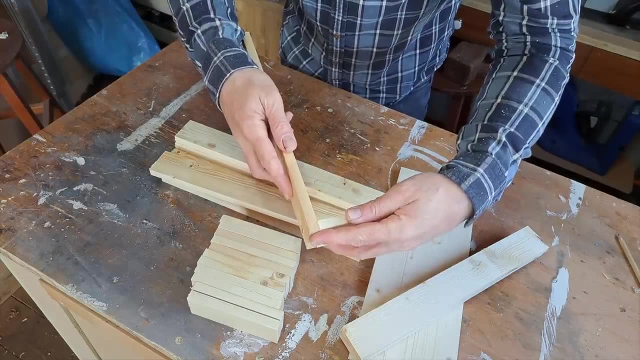 you're going to get. What is important is that for the sides and for the shorter end pieces, they are paired off with as close as you can get to being identical partners. I used a stop block on my crosscut station and instead of butting these together, we're going to route in a rebate into the ends of the. 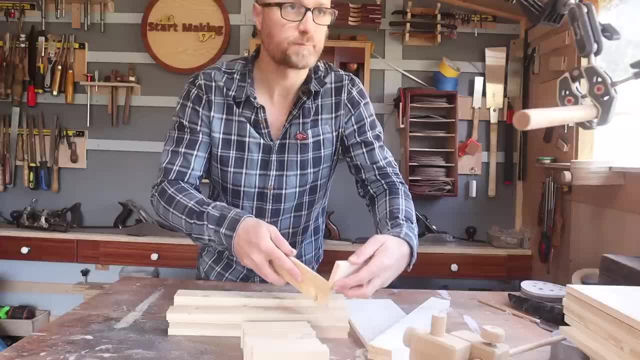 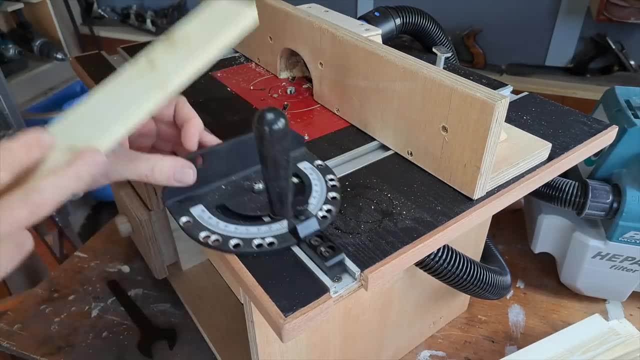 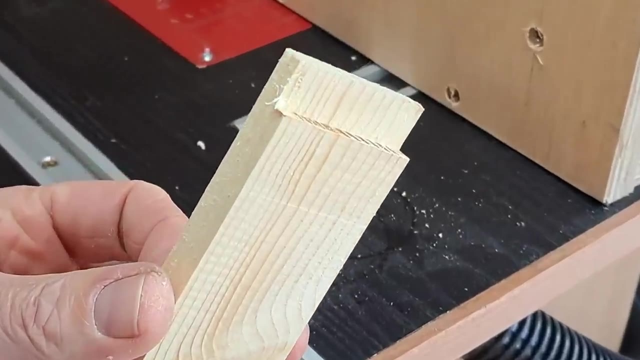 longer pieces that the short piece is going to sit in, And once we've done that, we can glue them up. I'm hoping that the router table is going to make my life a little bit easier here. The next thing we're going to do is: 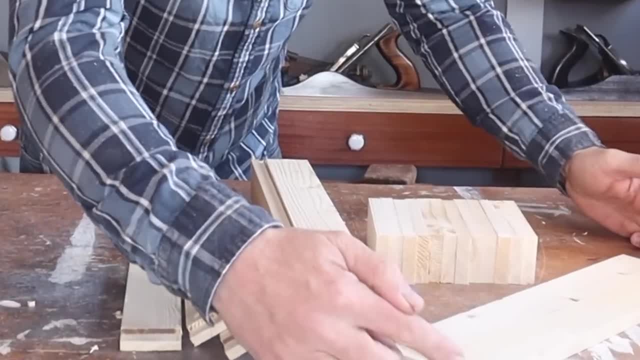 check that the two rebate lines are accurate. Once you've done that, it's dry fit time. After the dry fit, glue fit time, And after that we're going to work these up with some support because they're standing, And after that we're going to glue them up. 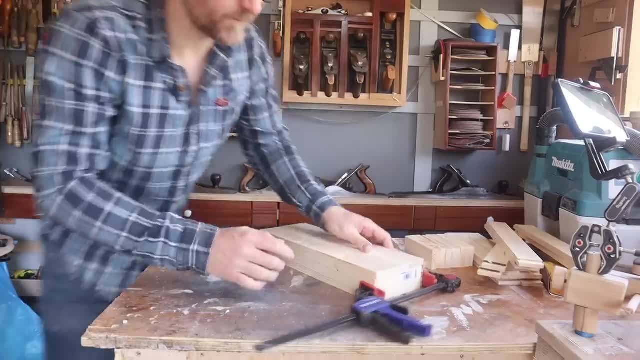 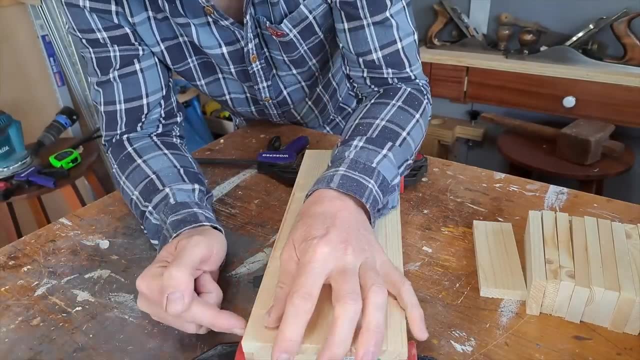 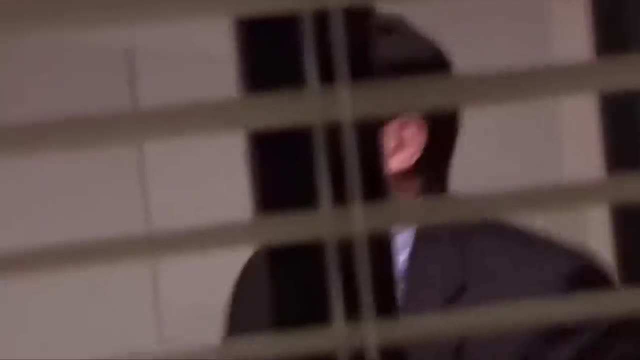 at the top and bottom, and we're nearly there and this is why we do a dry fit. check your tops against the bottom as well, because mine, I've got a little bit of the side sticking out by about two to three mil, if you get that really simple. 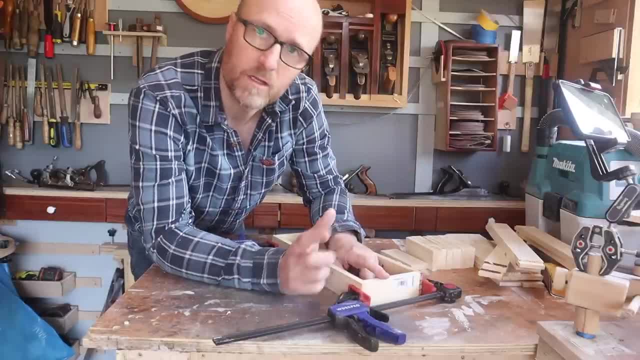 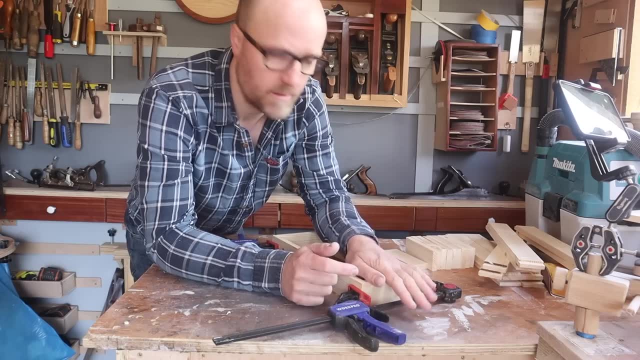 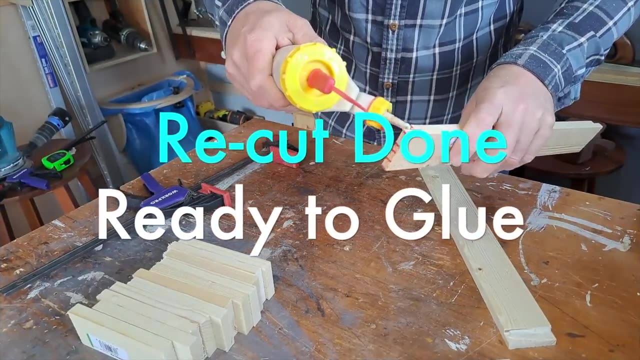 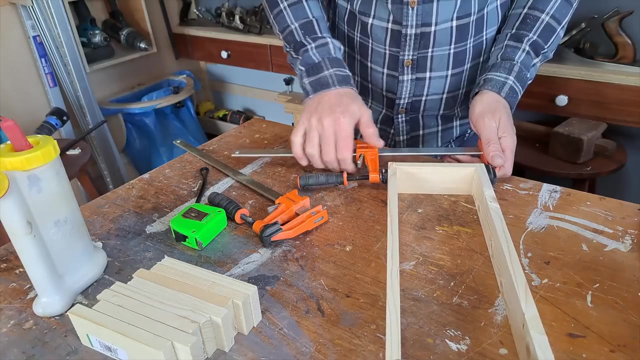 all you got to do is take these inner pieces and just skim off the distance. that's different, don't worry. these things happen in a build. I'm not going to hide my mistakes. that is just me measuring wrong, probably adding up wrong as well. once you're confident that the glue has gone off enough on these, the next thing. 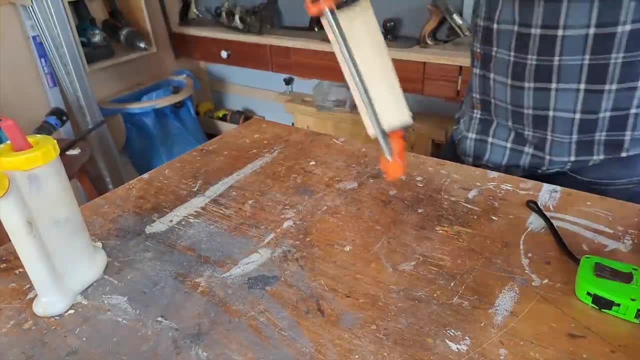 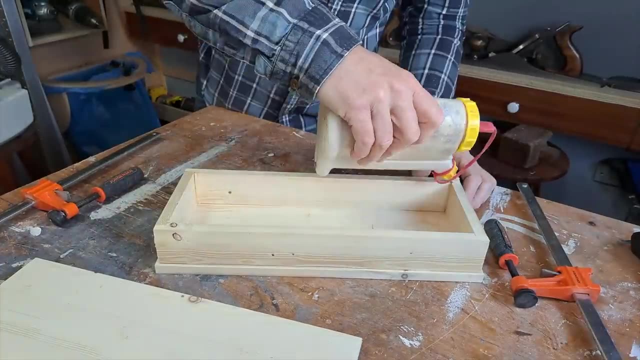 we can do is take the clamps off carefully and put the lids on. now, if you're worried about the lids denting and the bottom, because it's pine- it's quite soft- maybe put a little bit of glue on the bottom of the bottom and another piece of wood between the pine top and the clamps, starting to look a. 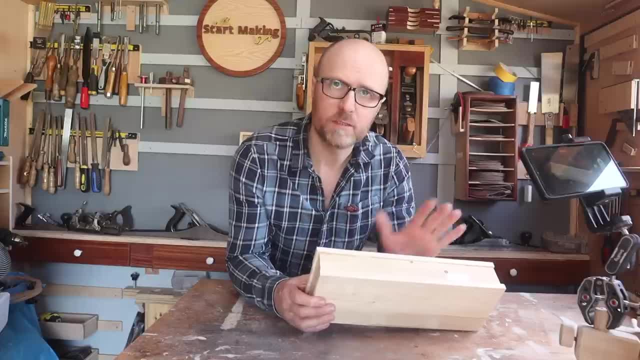 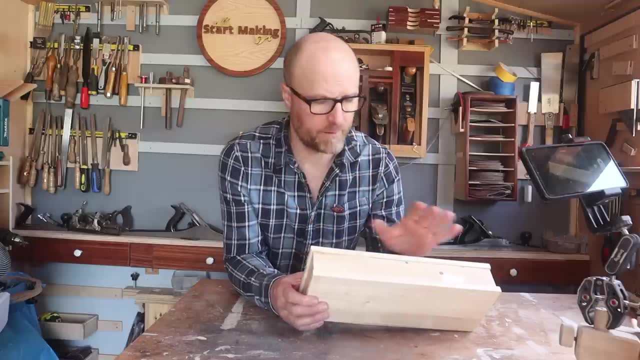 little bit like a box now don't worry if it's still a bit messy. everything we're going to do now is to clean it up and to get it looking really good. like anything in woodworking, there are multiple ways of doing anything, and this is no different. what I used to do before I got a router was I would just use a. 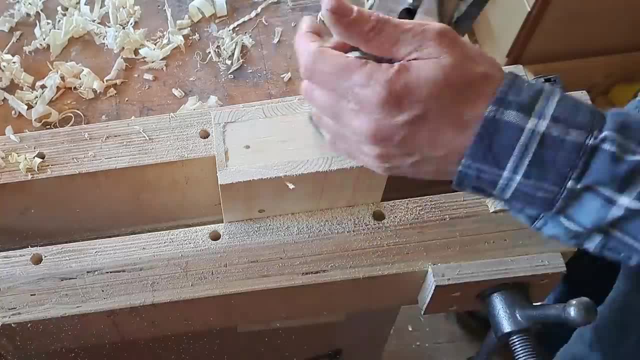 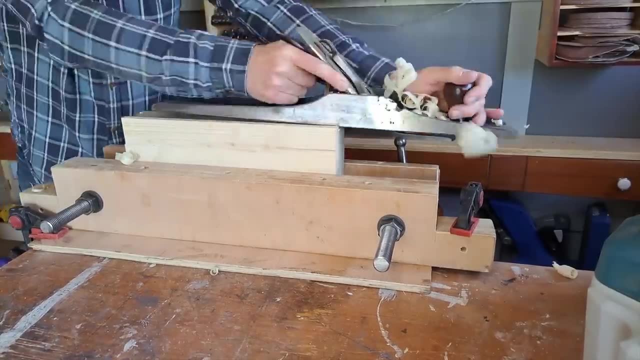 flush cut saw to take the two edges that are overlapping here, the excess from the top and the bottom, and then after that along the long grain I would plane it and along the short grain I would sand it. and that was a hard work way of doing it, especially if you're doing it in bulk. 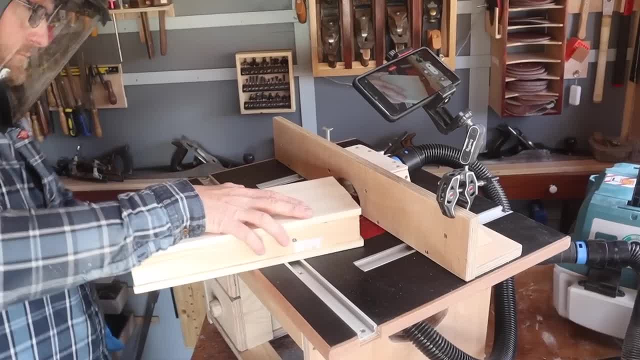 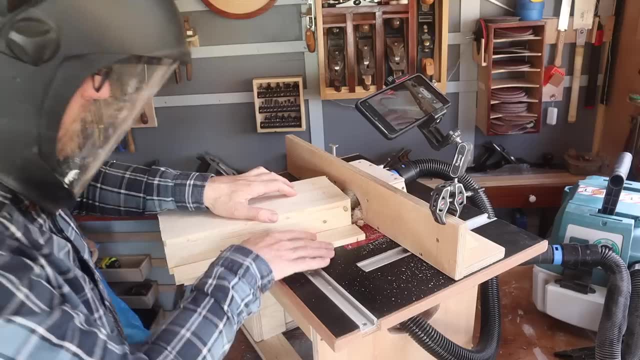 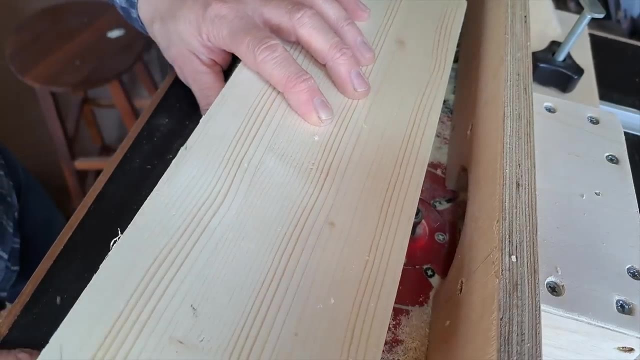 but now I've got the router table I'm going to give it a shot with a flush cut bit to see if that works. if it doesn't, I haven't lost anything. be careful of tear out. do the long grain first, because then you can cover any tear out with a chamfer on the side grain and take it nice and 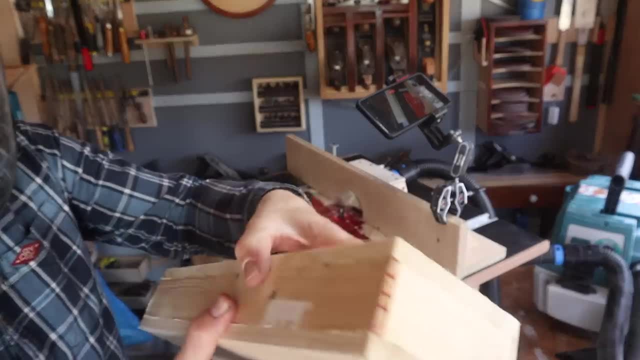 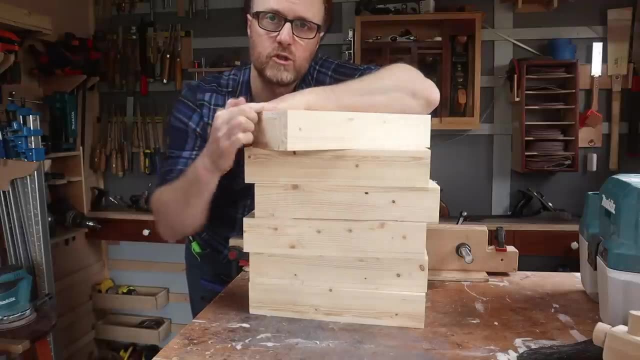 slow. don't try and take it off in one pass if you're not comfortable. what we're left with now is six boxes, but it's not a box if you can't get inside. so next thing we're going to have to do is chop the lids off. don't cut it too close to the top that you've glued on here, because otherwise 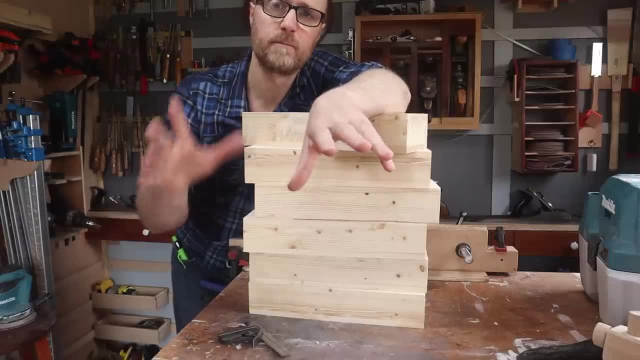 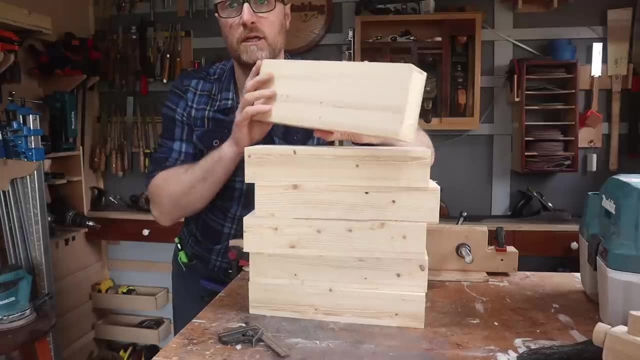 wood movement won't be supported. as for how you cut them, that's up to you. if you have a table saw or bandsaw- you're laughing right now- because that is super easy: pop it up on its edge and just run it through the bandsaw or run it through the table saw- a couple of ways. 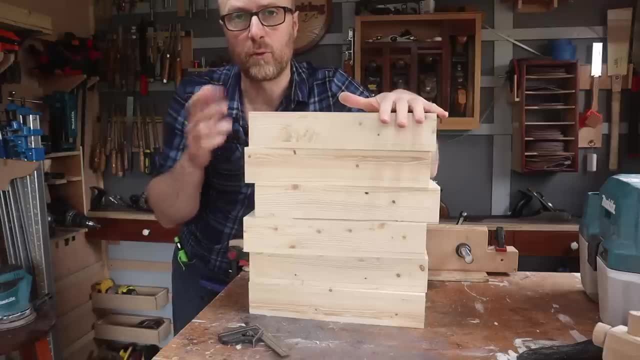 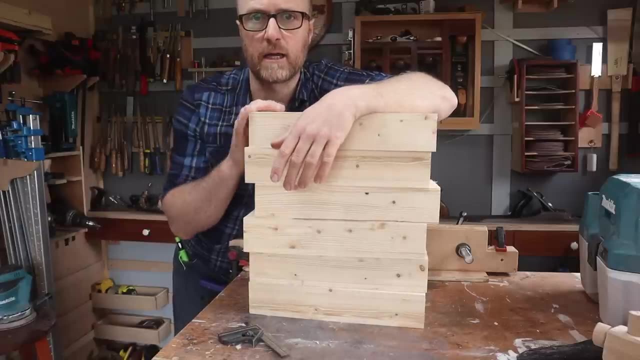 remember, if you're doing the table saw and you're cutting halfway through, support the bit that you've cut so it doesn't close up on the blade. just a couple of wedges in there. we'll sort that right out. so let me show you how I'm going to cut the lids off these. we're going to use a Japanese. 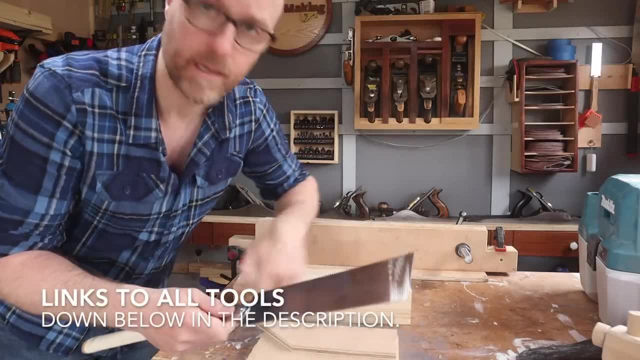 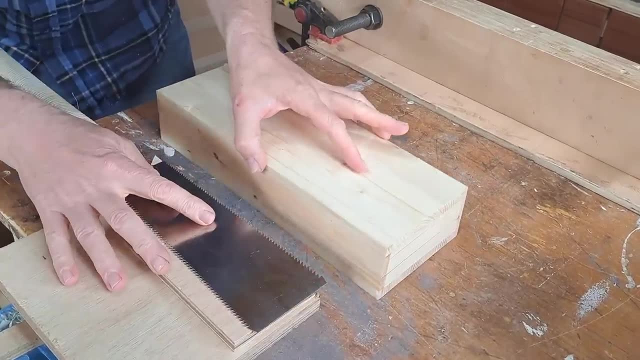 flush cut saw. we're going to use the rip cut edge because we're going along the grain, not across it, and we're going to put wood underneath the saw to the height of that line, which is give or take exactly a quarter mil plus a half mil piece of plywood. what we need to do is stick the. 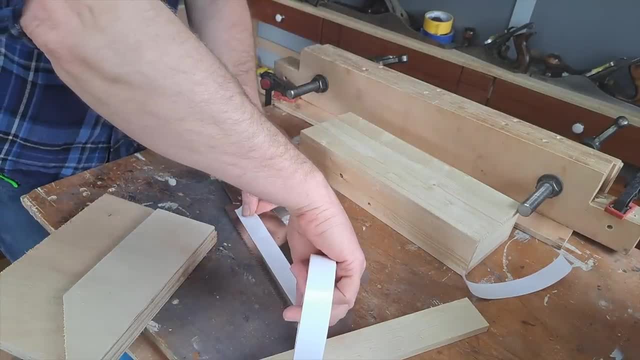 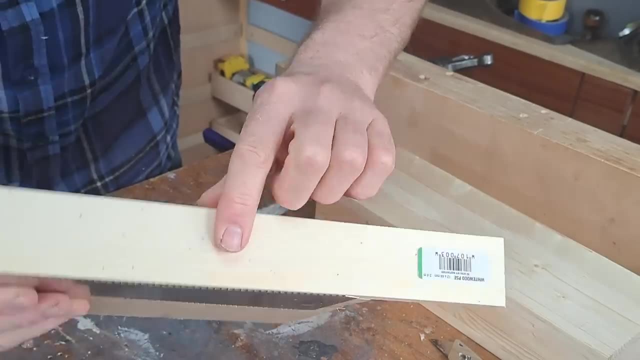 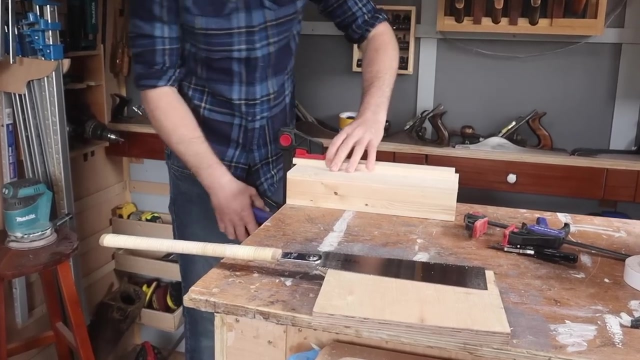 lids to the back of the saw so that it's raised up. we're going to reference off the bench heavily. we're going to set them back by the width of a piece of the scrap wood that we've got. don't go all the way through. they're very close, but you're going to leave one mil left on there. 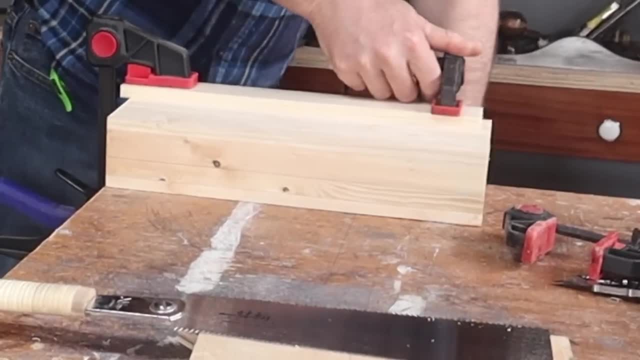 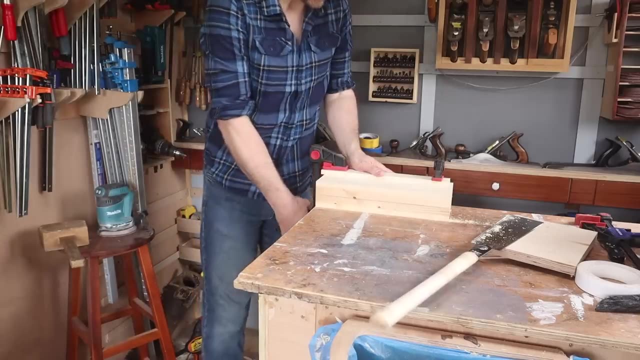 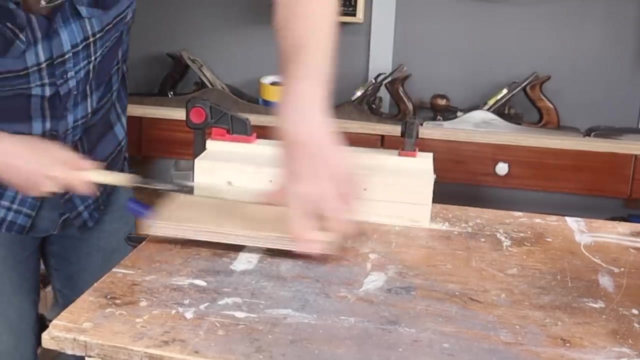 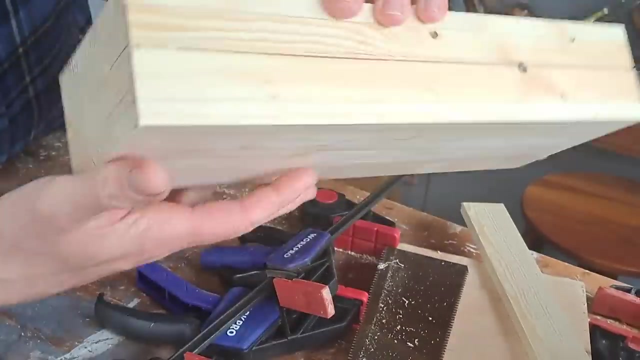 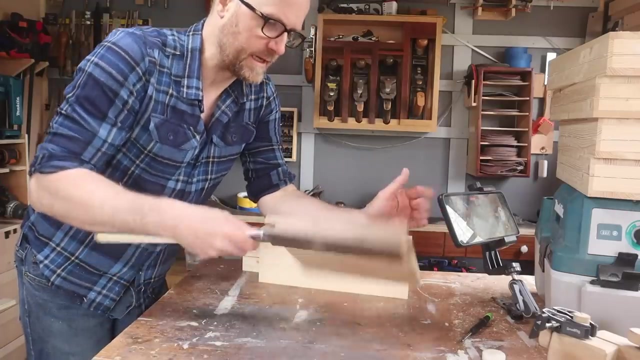 to support the cut all the way around. and then we do all four sides the same way, a method worked out perfectly. you can see the seams line up absolutely great. missed the line by a bit, but that's okay. two tips: very quickly wax the bottom of the wood underneath your circular. 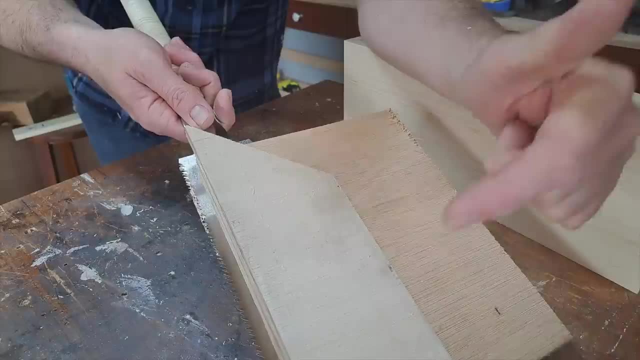 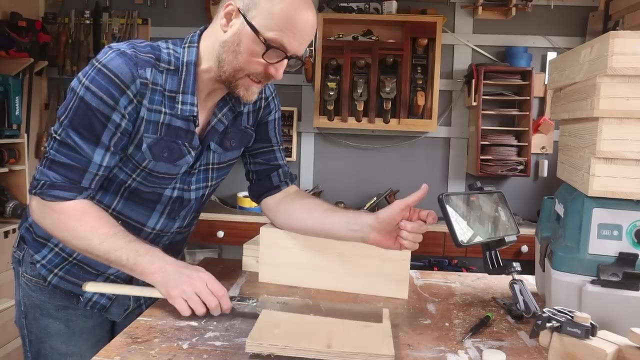 saw and have the least friction. this seems a little bit counterintuitive, having the bigger piece on the top because it might rock. but if you're careful, this is less friction. wax it up. secondly, clear your workbench. every time you've done a cut, don't let all the sawdust get underneath the wood because it will raise the 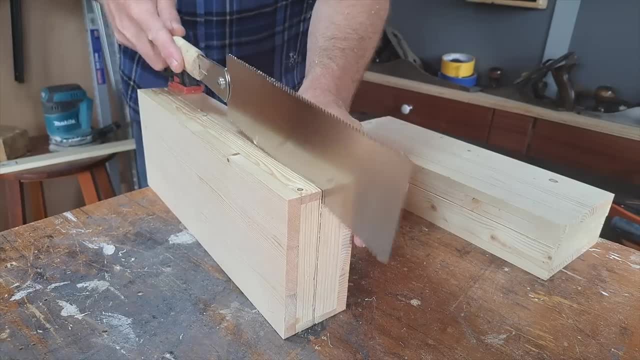 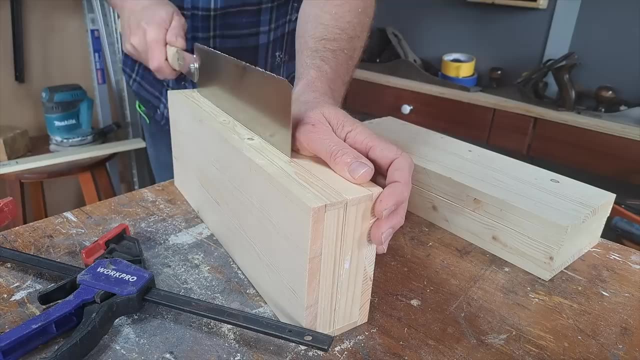 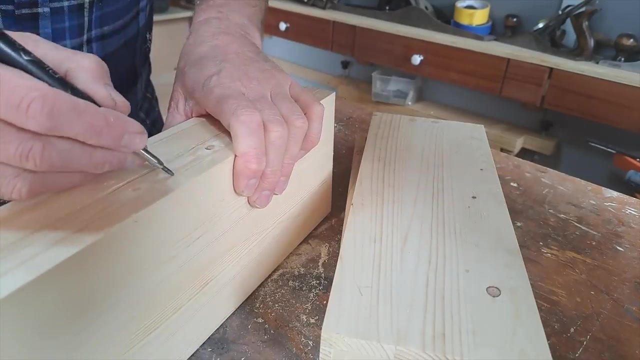 cut up and eventually you might go off that line. let's split these boxes up, mark them up so you know what goes with what. just put a little v on it so you know which is the front and which is the back, and then pop it to one side. 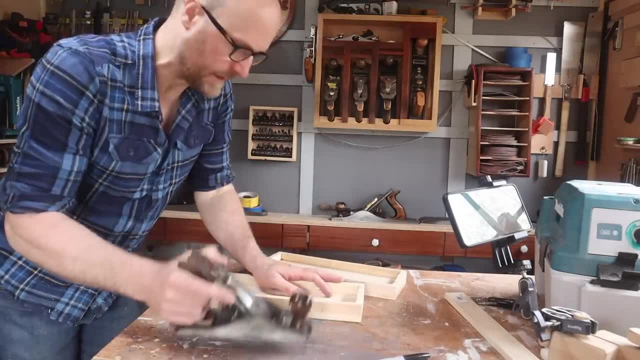 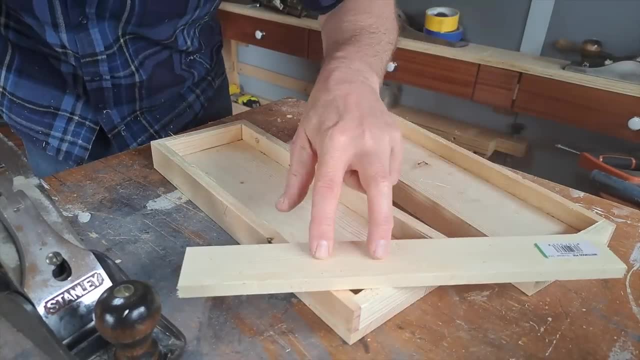 the best way that i know to clean these up is your hand plane. you could probably go about it if you glued sandpaper to a flat board and went about it that way, making sure that you're going across the angles and diagonals. personally, i like to have the plane and i like to walk it around the edges you've. 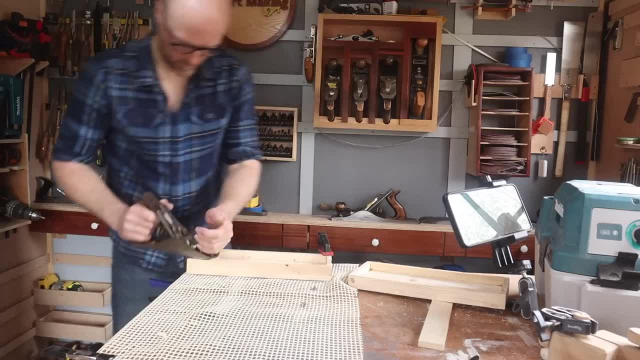 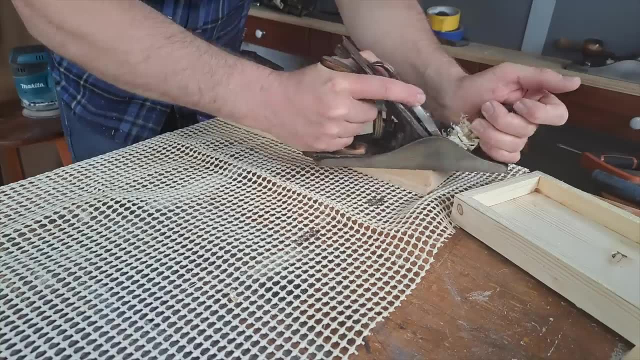 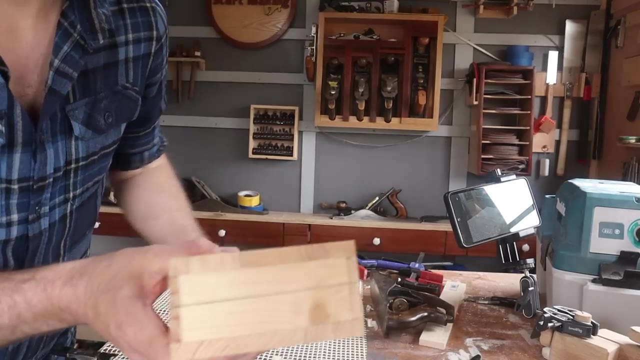 got a block plane and you prefer using that, go for it. have a little look at the grain directions when you start, because tear out is just going to mean you're going to have harder work now. none of that time have i tried to get it absolutely perfectly flat. if you close the lid and the base back up, see the tight spots. 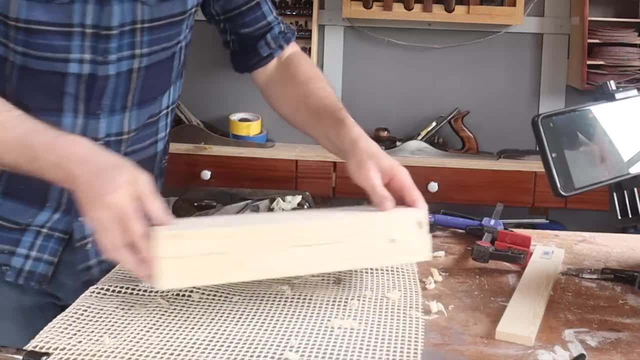 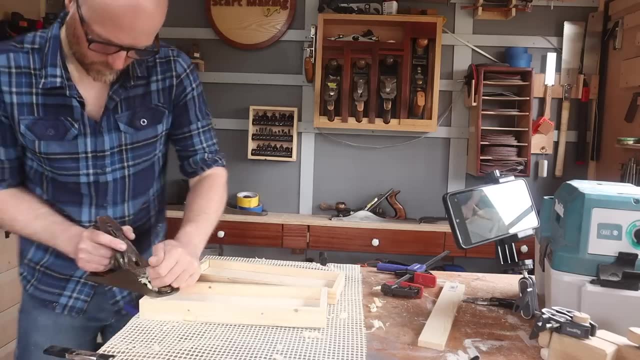 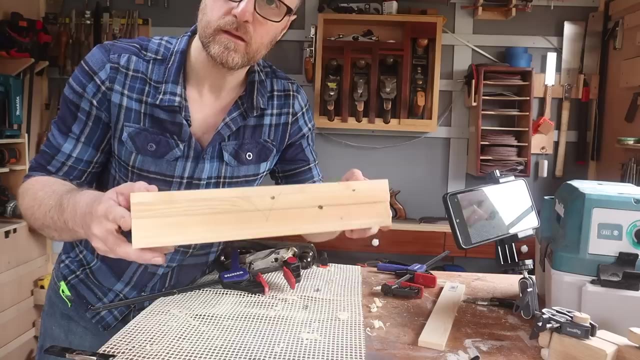 so then what you want to do is just take your plane and level off some of the tight corners, because eventually it will fit perfectly into place. then, once you're happy with the fit, do all the rest. you'll get better as you go along and it'll get quicker. then we've got a. 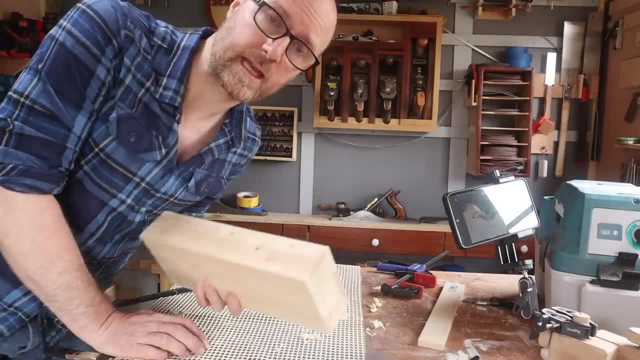 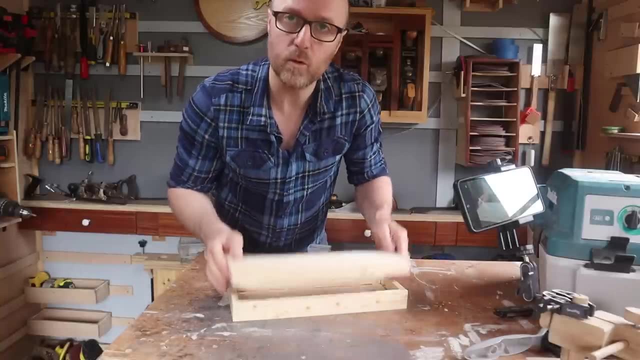 box that you can decide what you want to do with, and i'll talk you through that when i catch you up. one thing i will say is this doesn't have to be a hinged box. from this stage onwards, you can put anything you want to keep this lid on. you can put magnets in each of the corners. you could put 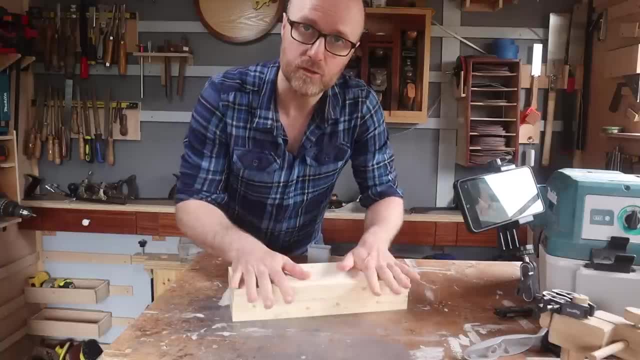 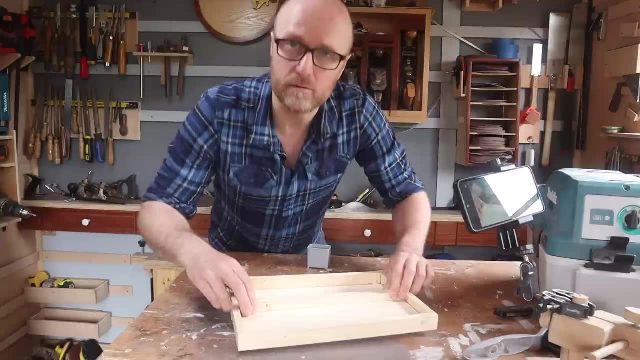 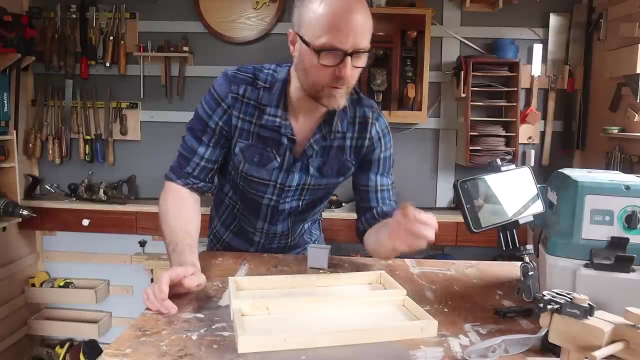 another layer of wood inside, slightly protruding, so it sits flush on top of it. you can do what you want. i'm choosing to do hinges just because you know what it drives me nuts and i hate hinges. maybe we shouldn't have done hinges anyway. that's part of the design. now i've got these small hinges. 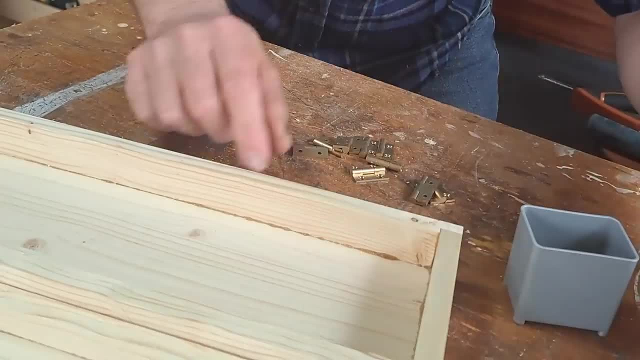 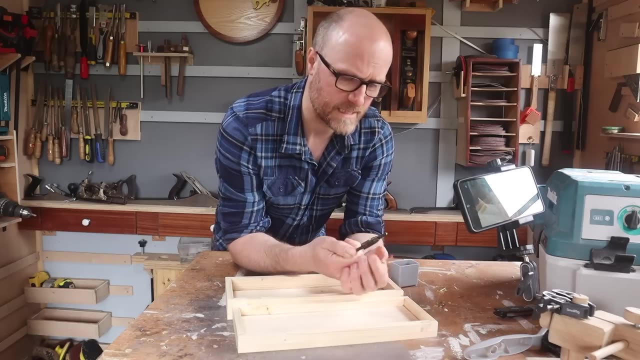 and i've got these smaller hinges. i'll leave those there. i'll leave them here at the back of the contents, but anyway you can become a hinge during this stage. some small screws and one of the priceless additions to any workshop: the centre finding drill bit. I'm not sure that's exactly what it's called, but 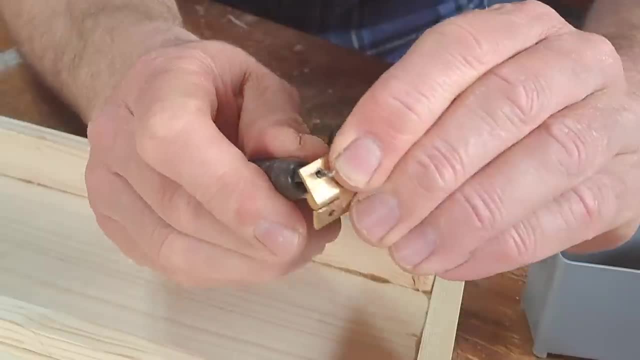 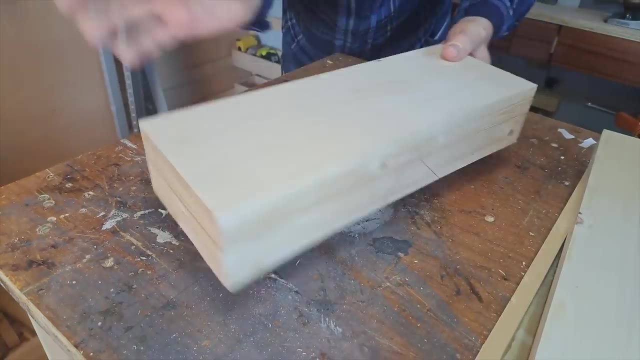 basically, when you push it down into this, it will find you the centre. There is a trick that will stop this happening. You see, it's flush on one side, not on the other. That's purely because one of the hinges I've set is around about a. 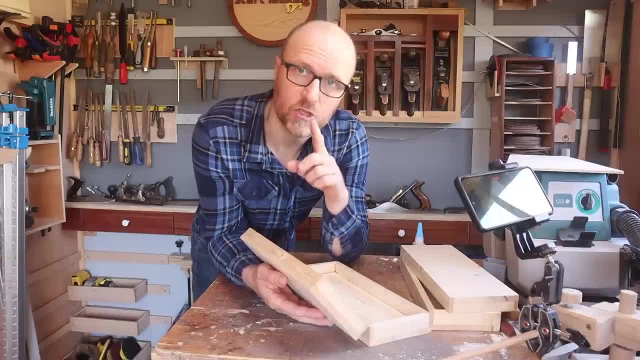 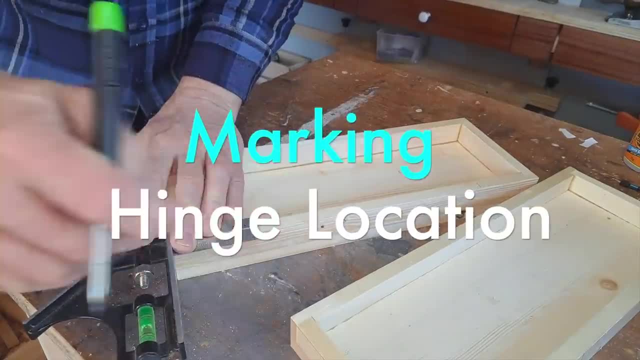 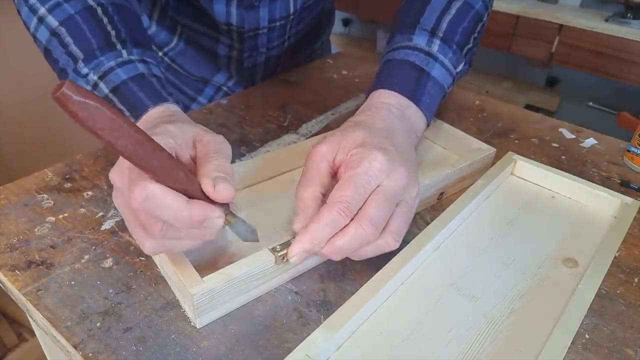 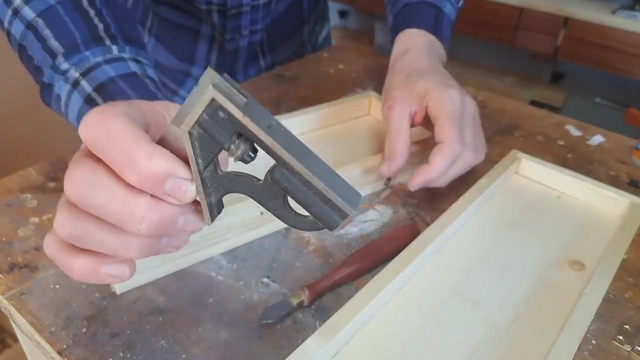 millimeter out of whack and I'm going to show you a nifty little trick that's going to help you get past that and make sure that your hinges never let you down. Seat the hinge and scribe around it, and then I've set my adjustable square to. 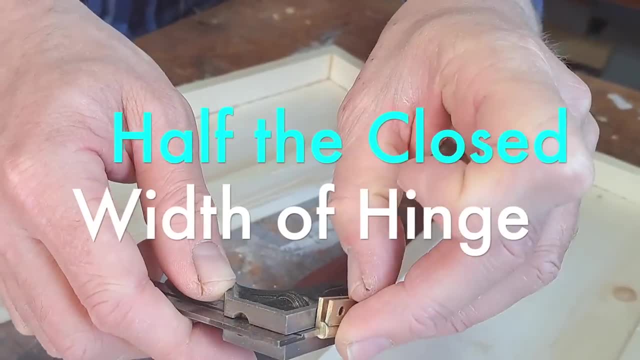 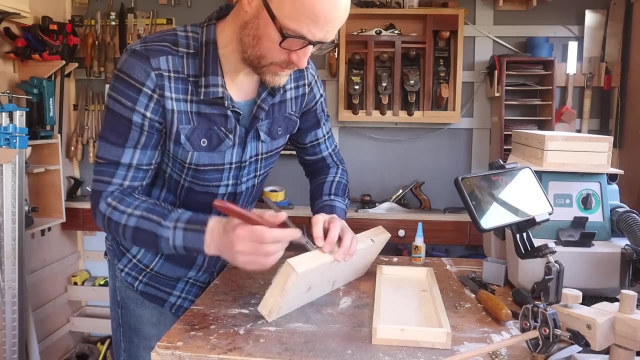 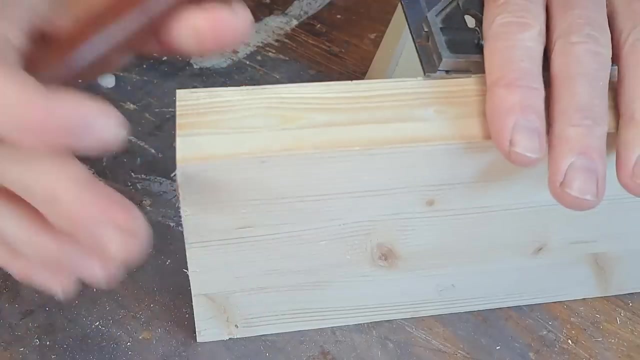 the half, or just slightly under half, of the total opening of the hinge. and that's so that I can scribe down the back and make sure that I don't go too deep. Follow the marking across so that you can see it on the back, and that's from the edge of your hinges, and then scribe. 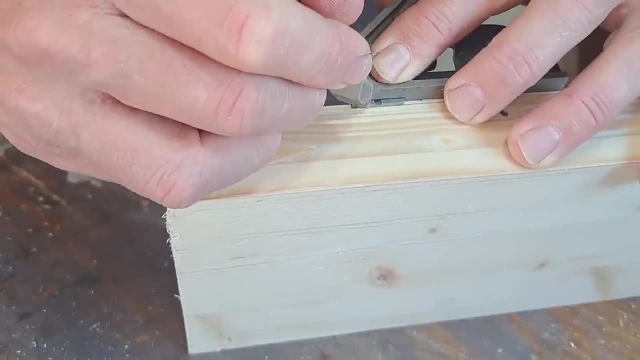 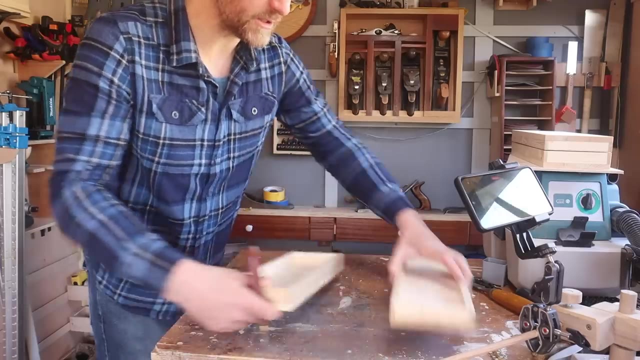 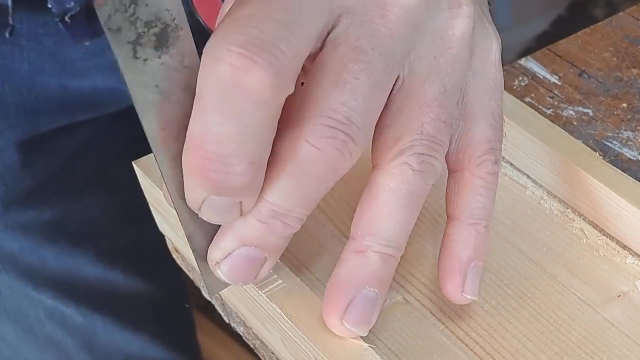 along your square so that you have a depth line on there. Then do that for both hinges. The next thing we're going to do is find our sharpest chisel and we're going to remove the stock. One thing to remember here is your. 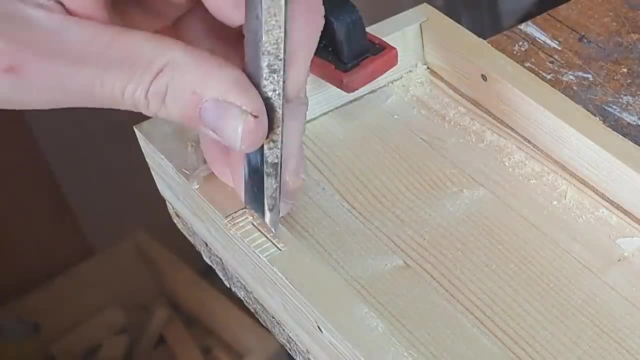 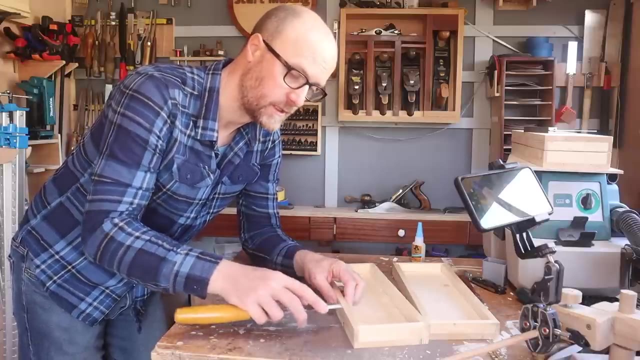 first time putting the chisel in. don't go straight for the knife lines that you've made. Come in around about a millimeter because I guarantee when you start hitting it with the mallet it will move across. and do the sides first, then the top. If you do the top first, it will split further than the sides You want. 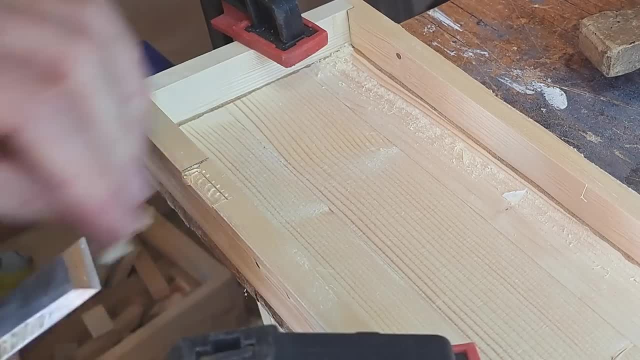 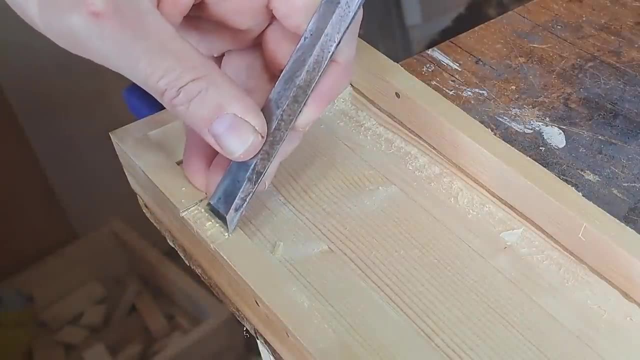 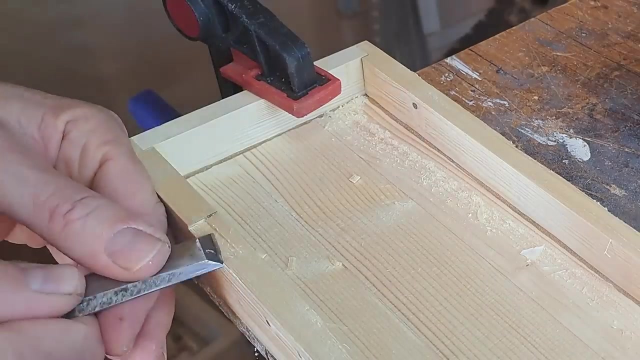 the marks on the sides to hold the top in place, and then after that, we just remove from the end upwards, being very careful not to over shoot and make sure that it's down to the right depth, Clean it all out, make sure it's flat, Super, super simple. Okay, so here's the start of the bit that's. 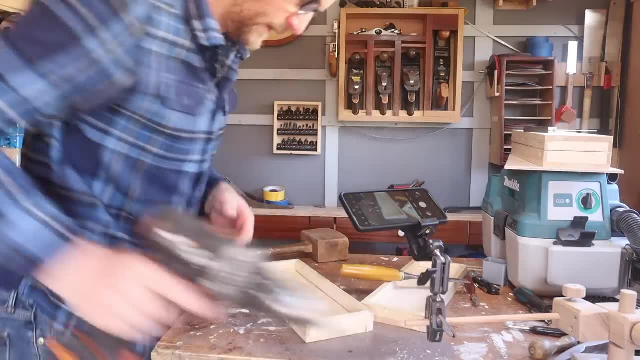 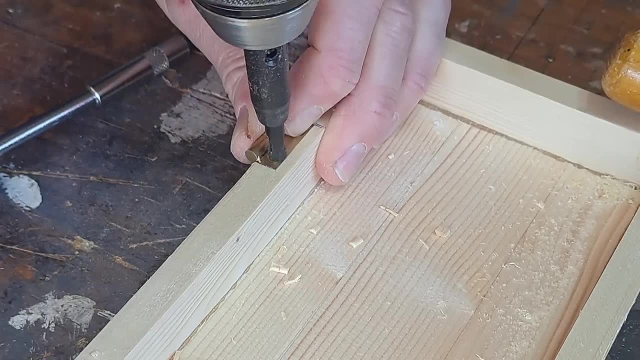 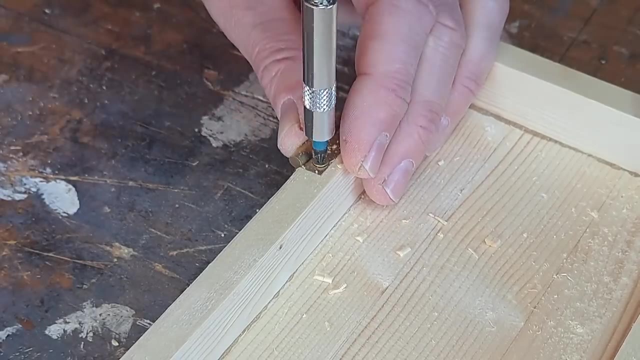 going to save you a lot of grief down the line. First thing you want to do is seat your first hinge and take your self centering bit. drill out the first one. pop a screw in pivot insert on this screw, using the barrel for reference to make sure that it is as 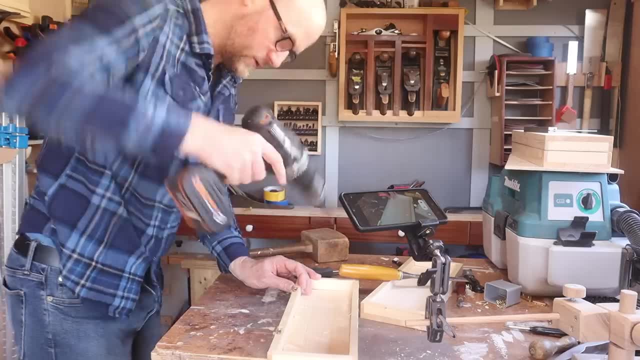 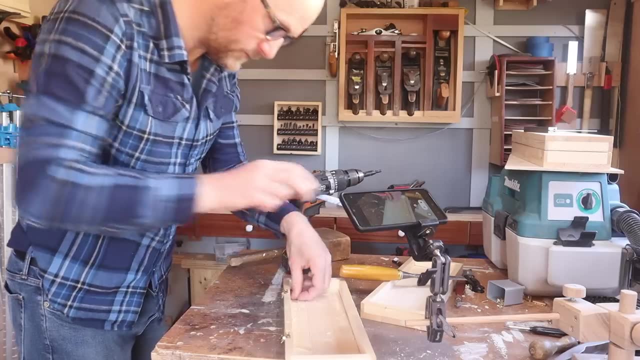 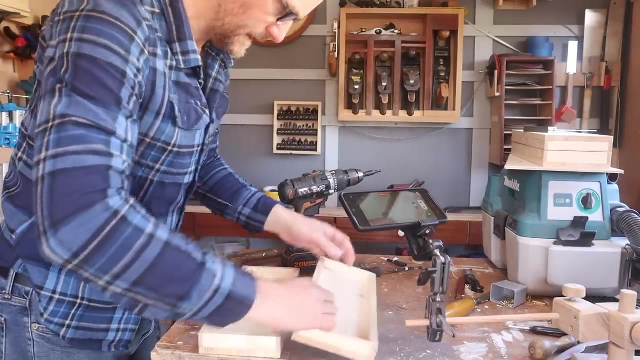 square as you can possibly get it, and then drill out another one Second, screw in and these two are ready to reference off on your lid. Now, normally what I would do here is I would put the lid next to the box and then I would just. 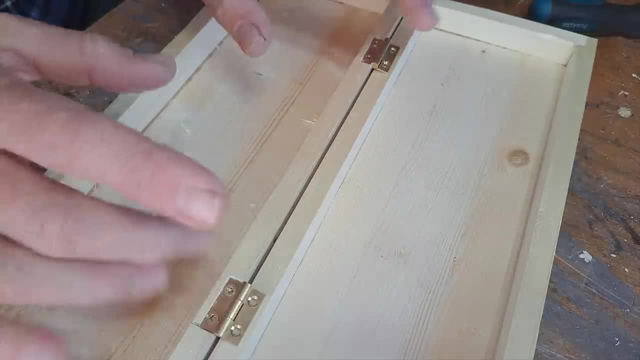 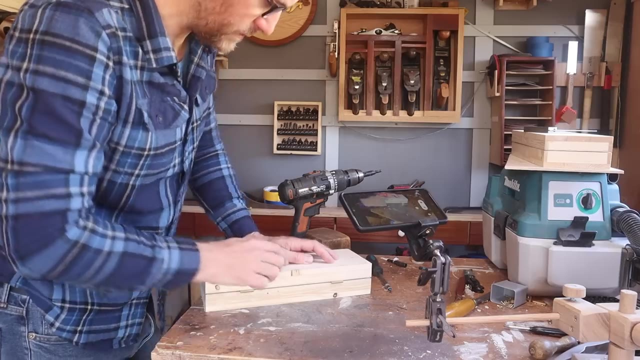 mark off one, hinge onto the other, and that's the problem when you're doing this. So if you start chiseling these out and you get them slightly off, whack, you can have the lid sitting on a skewer. It's a bit of an extreme example. 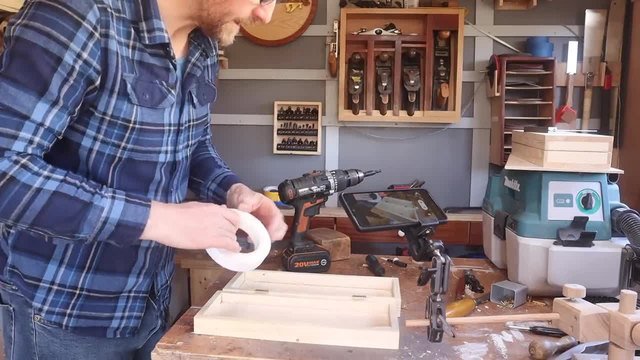 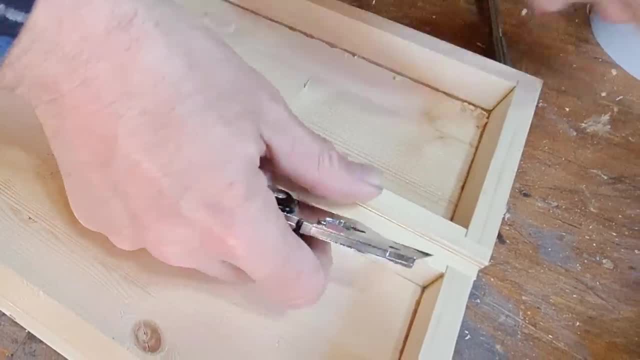 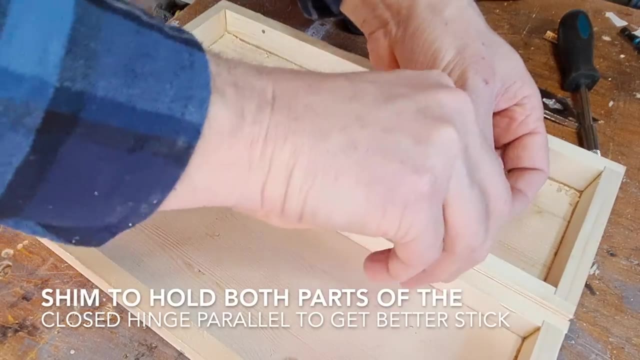 This is where we're just going to use a little bit of double-sided tape to help us with our job. Just pop it across the hinge, one on each, and then peel it off. It's worth popping a shim into the hinge to keep it flat. 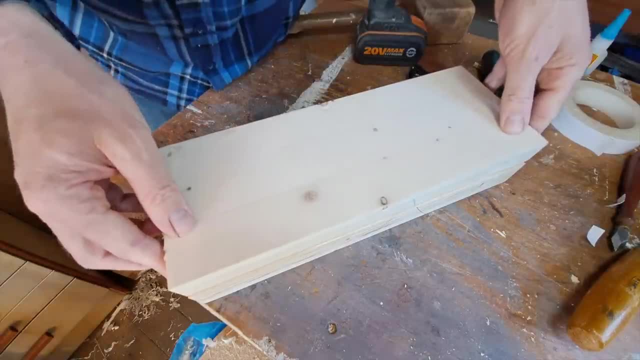 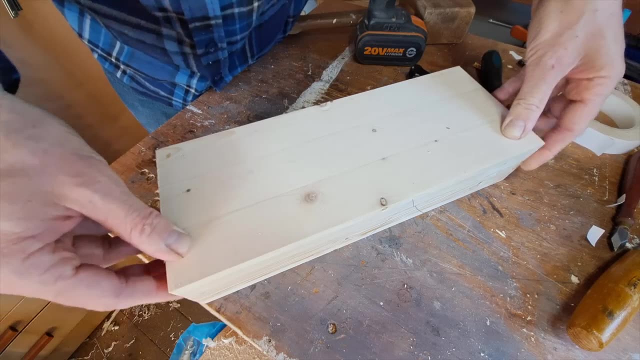 Anything that's a similar width to the gap base will do. Pop the lid, flush on the front. Try not to press it down quite yet. Make sure it's exactly where you want it. Flush on the sides, flush on the front and then. 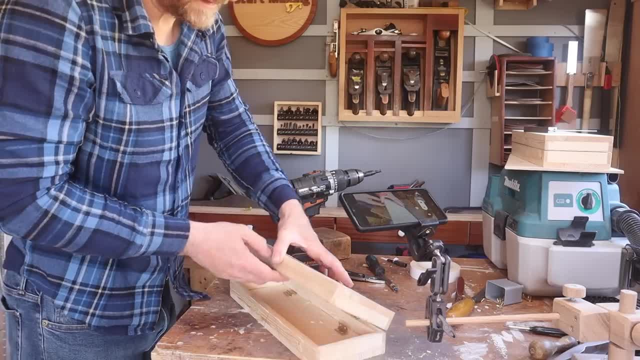 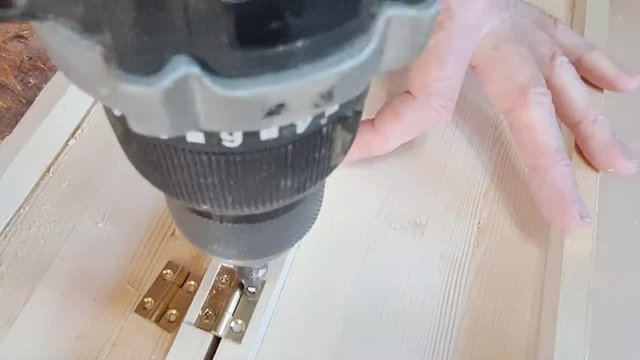 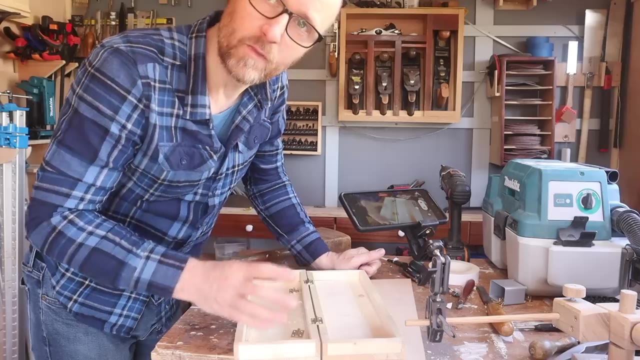 activate the tape with pressure, Moment of truth opening it. We're not going to do anything but drill both holes on them. Any mistakes you make now, those holes will pull the hinges to exactly where you want them, and that's the trick. 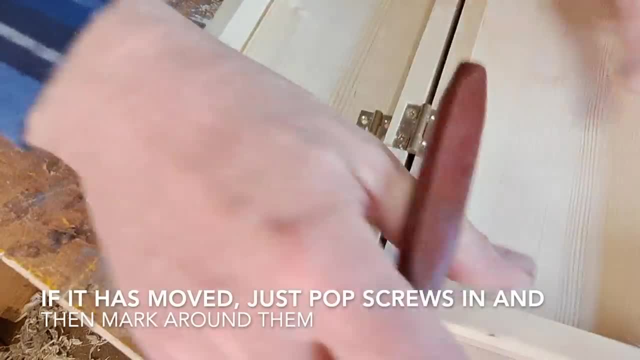 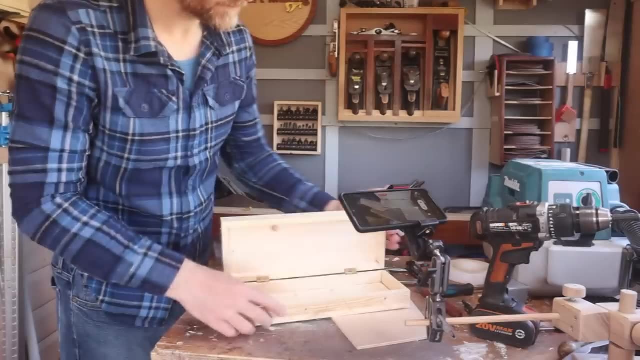 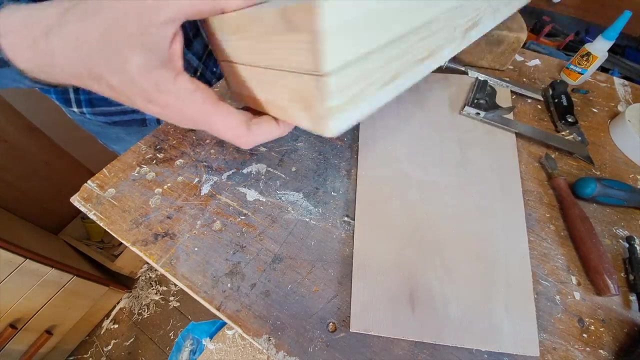 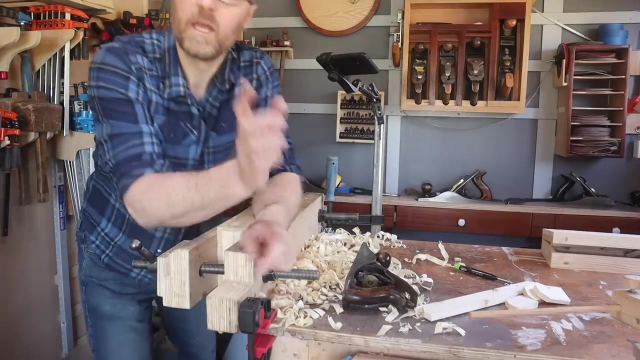 If it hasn't moved, you can mark these in position, Mark them, chisel them out and then seat the hinges. That is as close to square as someone like me is ever going to go Makes it so much simpler If, once you've got them closed, you're noticing a mil difference. 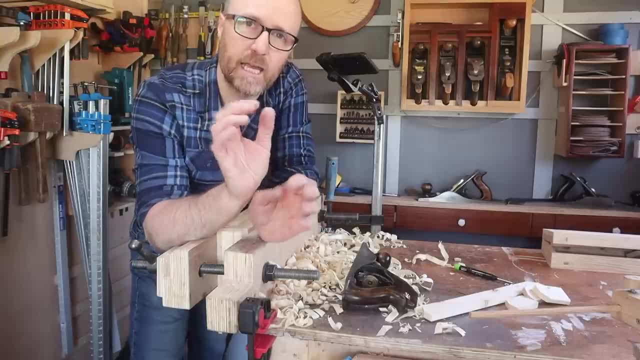 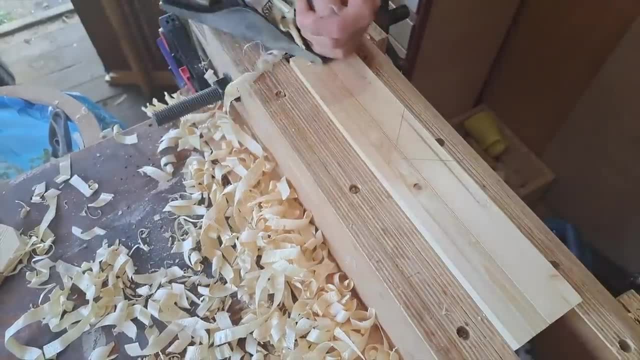 about nothing. big big ones. you've got to reset the hinges. but if you're noticing a very small difference where the top meets the base, this is where I just like to pop them in my vice and very carefully, I like to just even it out and just take the overlap off so at least at the front forget. 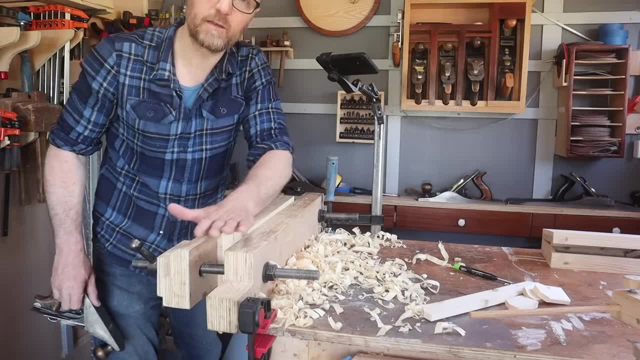 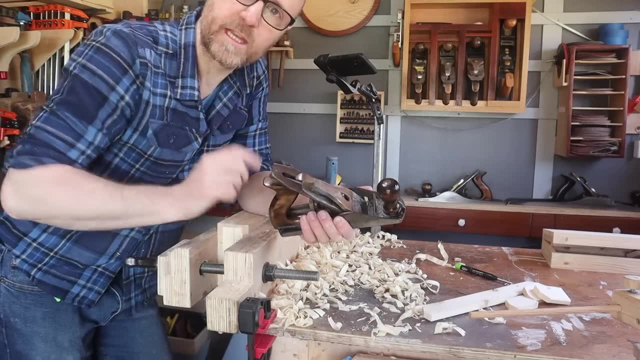 the back, at least at the front. they will then be absolutely flush for anybody looking at it. it's really easy, just make sure you take your time. but once you've done all of this and you've got the boxes square, we can then set the inner pieces for the dividers we're going to be using. 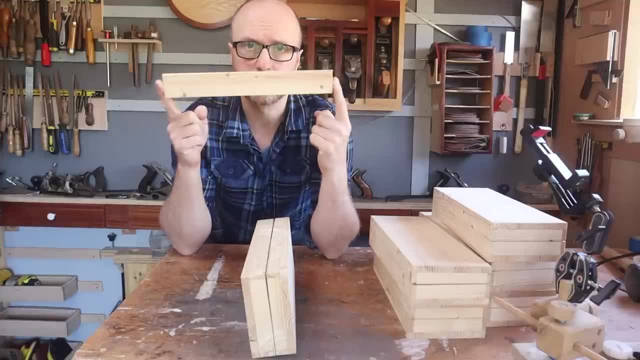 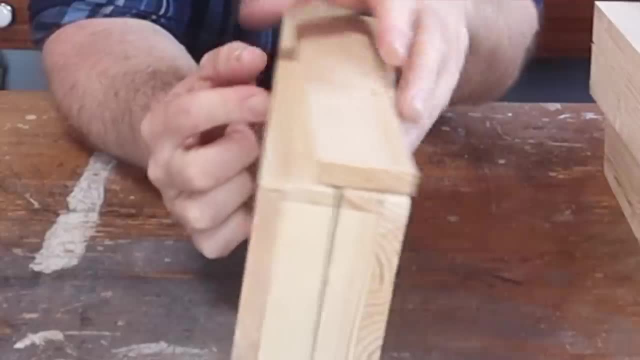 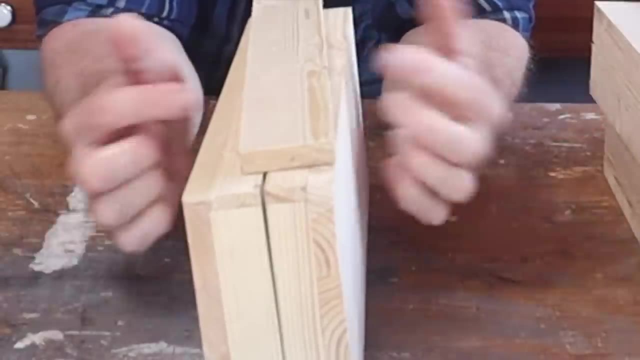 the same pine stock that we had to start with, and it should be the same width as the sides, because that's what we made sides out of. however, when we cut the box in half and planed it, we lost approximately two or three mil, not as much as if we use a circular saw, but what we need to do is: 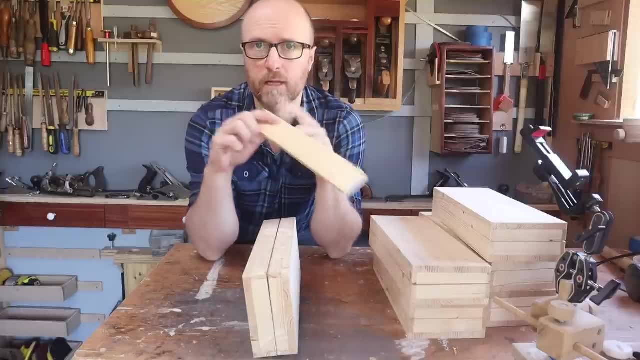 make sure that when we're cutting these, we also take off two or three mil across the top. you don't have to watch me do it. what I'm going to do is I'm going to cut the top and then I'm going to just hand plane them all down so that when they're glued inside they don't hold the box. 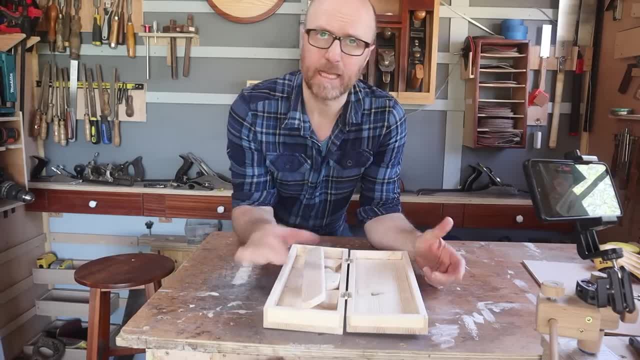 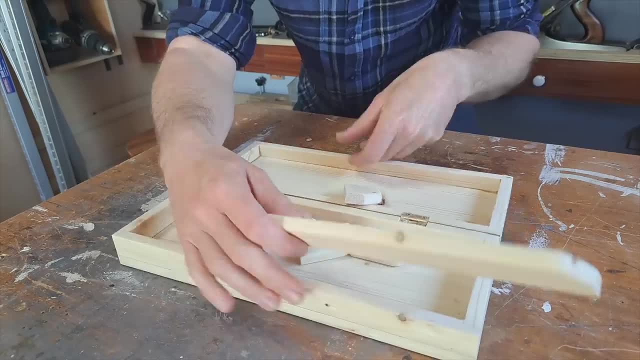 open. what I didn't think you'd be interested in seeing is the sanding, basically all of the smaller parts inside. I've given them a sand, I've rounded over the edges too, and they've all been cut to size. this one, for instance, will have the centerpiece sat in and then 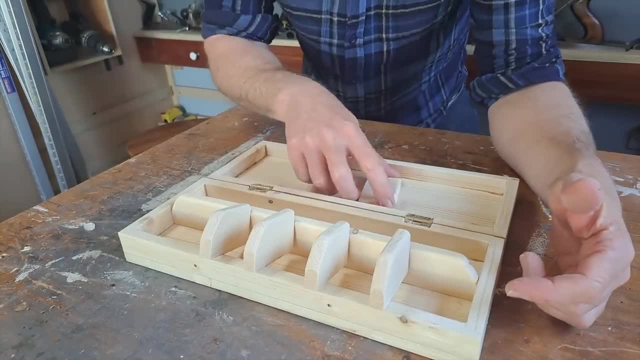 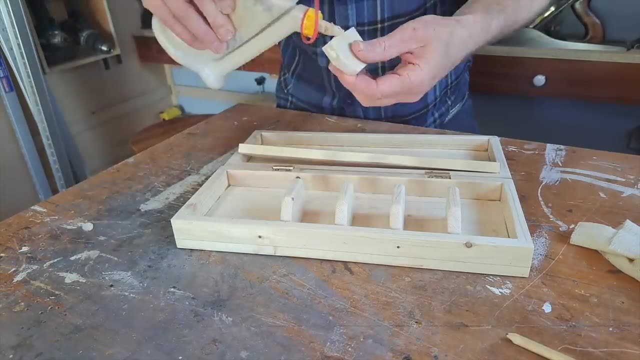 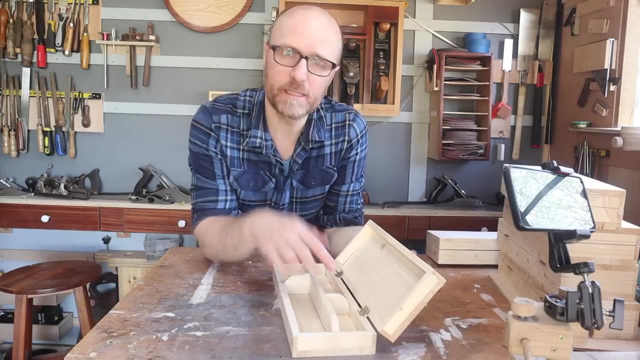 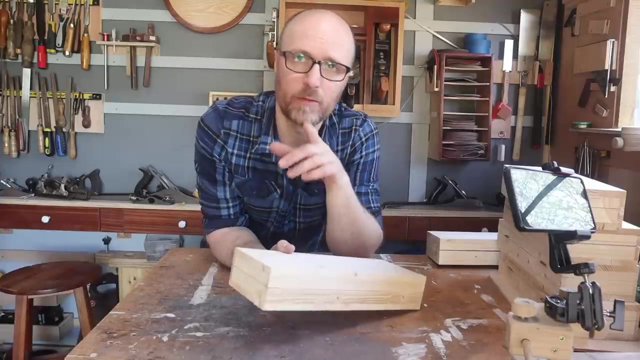 we'll have five dividing pieces across the front, one down. so with the internals in place now, the inside of this box is pretty much done. we haven't done a lot on the outside, and that's what we're going to address now. now, this is really as far. 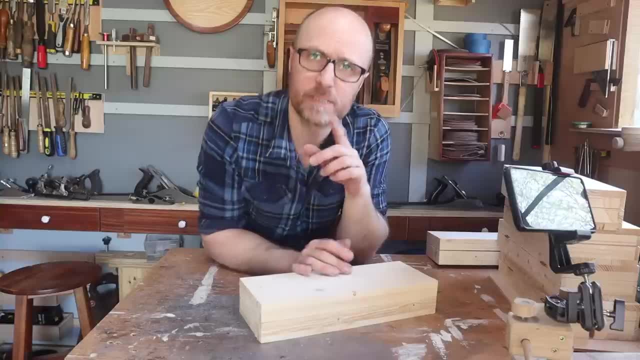 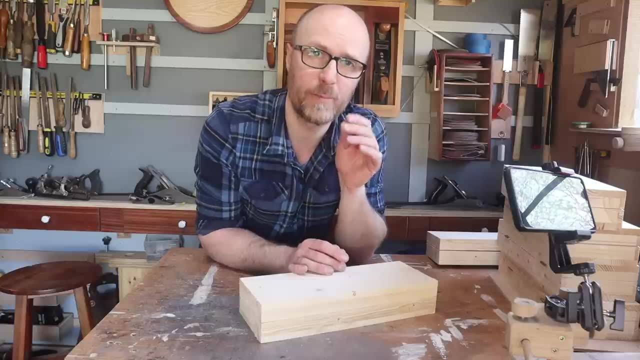 as you want to take. it is the honest answer here. if you're planning on selling these, though, one thing I would say is: as personal as you can make them, the better, and also, I'm going to show you a way that's going to give you flexibility, so that, if you're selling them and you have numerous, 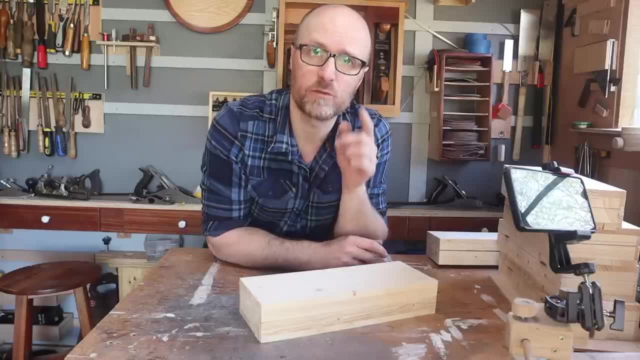 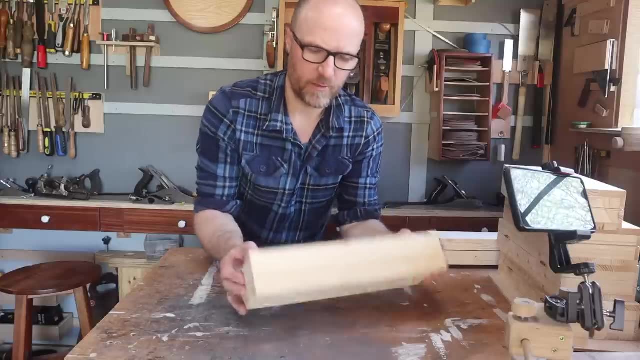 of them, you can offer something that's a little bit different to every customer that you talk to, and I think that is going to be a really interesting selling point for you. the first thing we've got to do, though, is neaten up all these edges. they are a bit blocky for my liking. 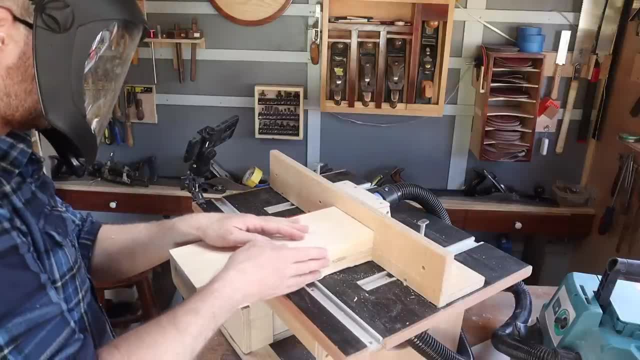 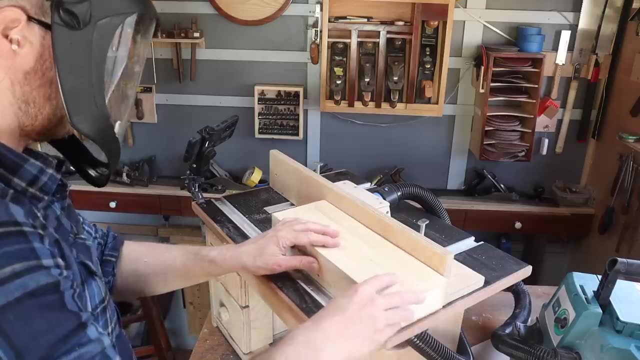 now I'm going to use my router for this because, well, I've got it. I'm then going to put a very small chamfer or a round over on the bottom- could very easily just use a plane and chamfer as deep as you want into the sides and then, if you want, to round them off with a sander. 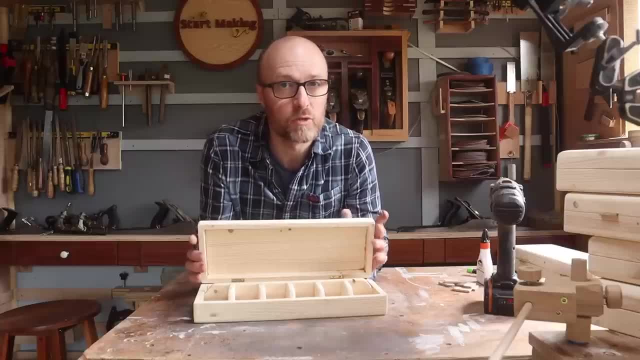 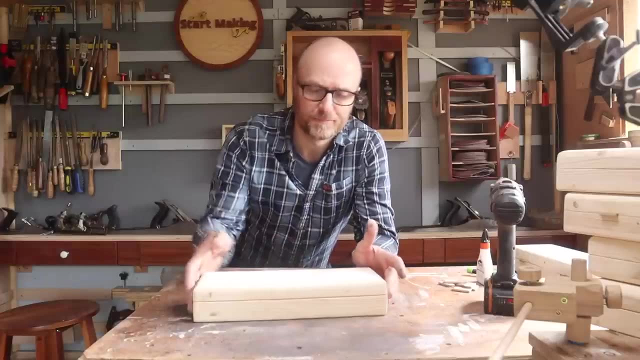 do it that way. I think this is the best and most important step, and that's personalizing. what I like to do is just put a feature on here that will help it stay closed. now. you could put it on the front, but it's going to be off center and I don't like that, and I think that's the obvious choice. but 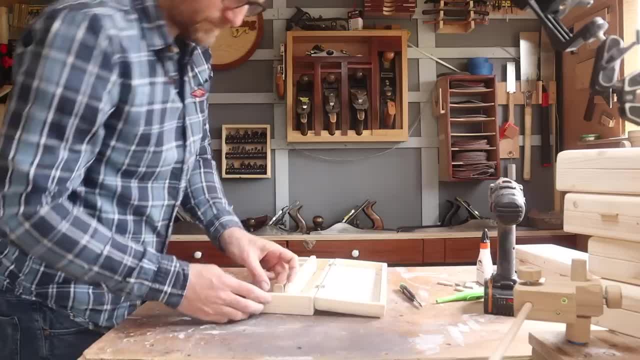 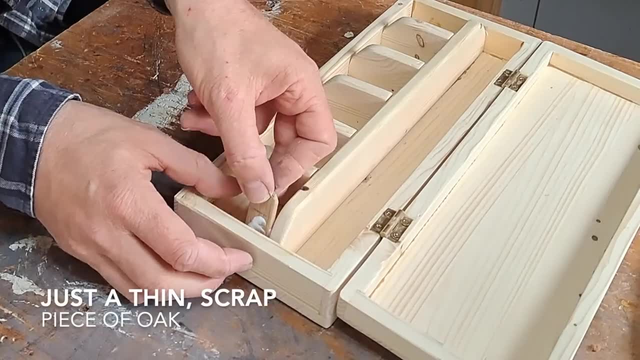 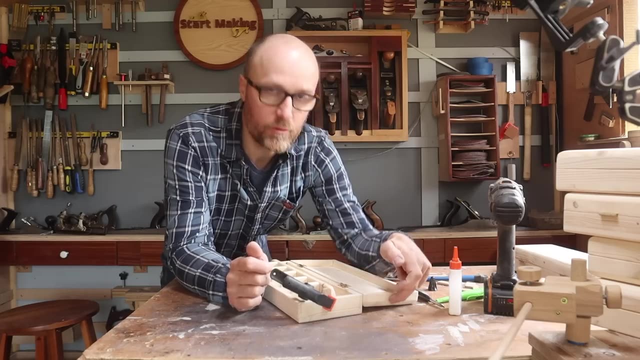 what I'm going to do is put something on the end here that's not only going to keep it closed, but it's going to be an interesting and very good way of customizing it when you are selling the box. well, the first thing that we'll do next is is just a little tab of wood that we are going to drill. 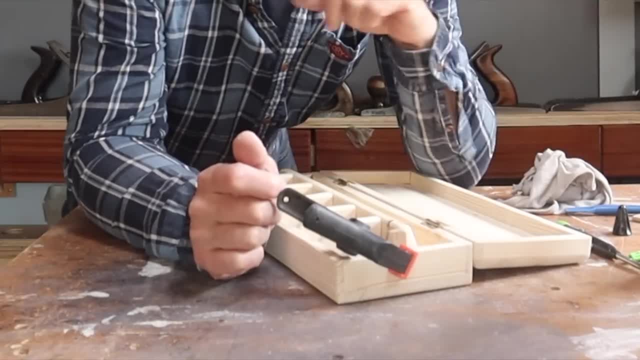 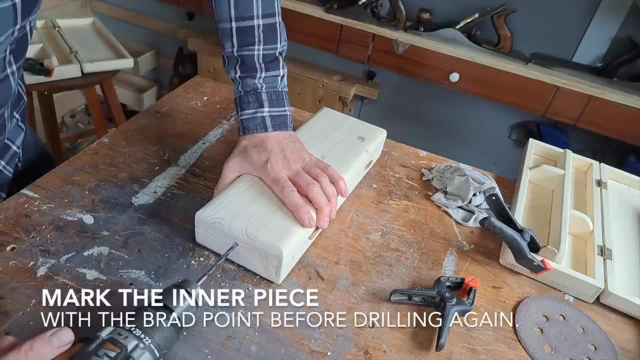 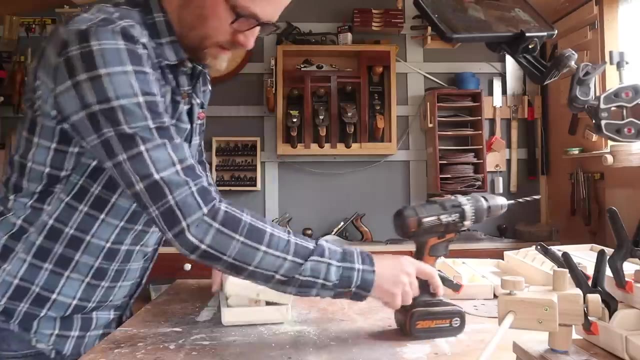 through the side of the top, through the tab of wood, and then we're going to place an interesting little dowel feature through it to lock the box together. then we have to drill through the outside box and the inside peg. that is your locking hole. so now you test it with one of your pins. make sure. 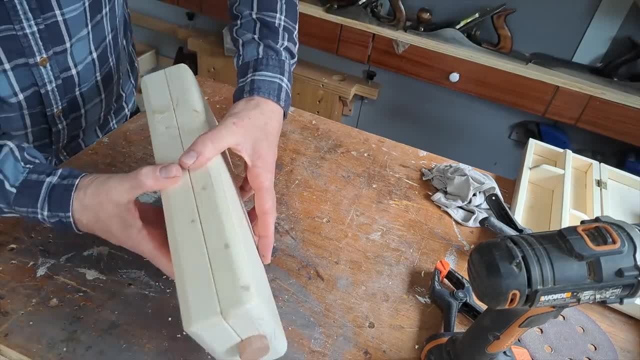 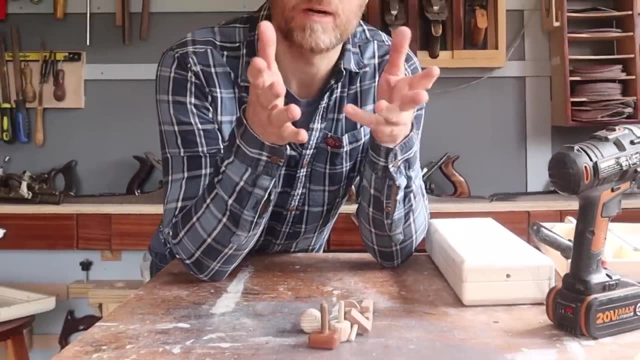 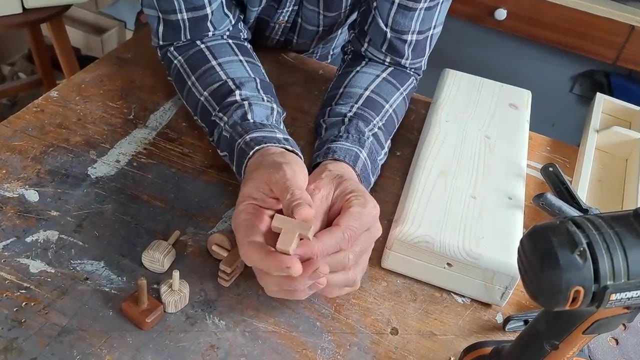 it goes through and that and is a lovely feature. Now I said about offering people a choice and customisation. I would make an alphabet and I would have all the popular letters and I would have at least three or four of some of the most popular ones, because 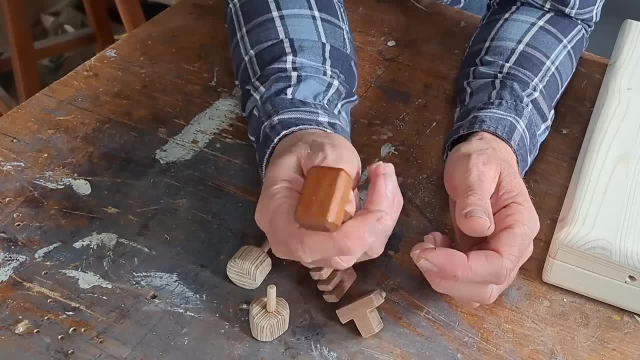 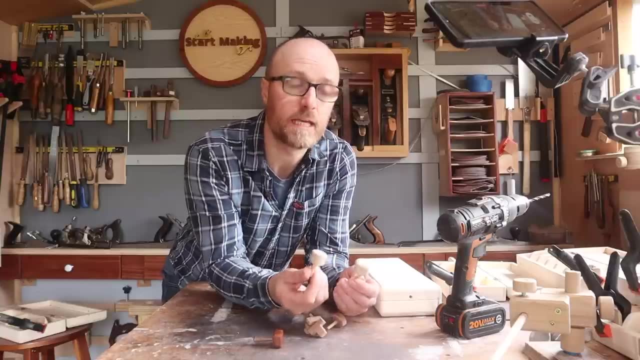 people's names. I'd have stars, hearts, Thor's hammer, Don't know why, thought that might be interesting and it's really simple. I'd make some out of dark wood, light wood. I've even done some out of the herringbone ply that I had left over. 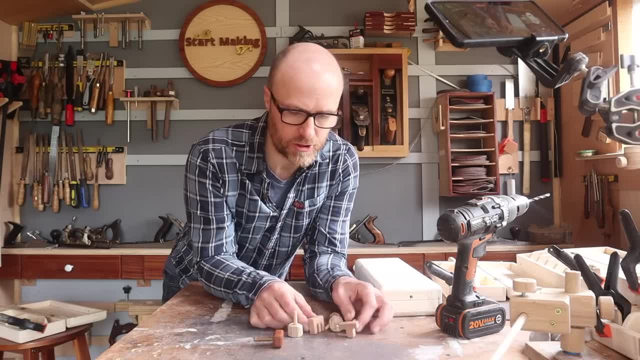 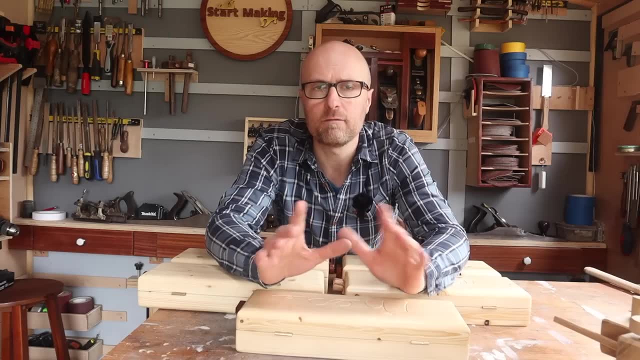 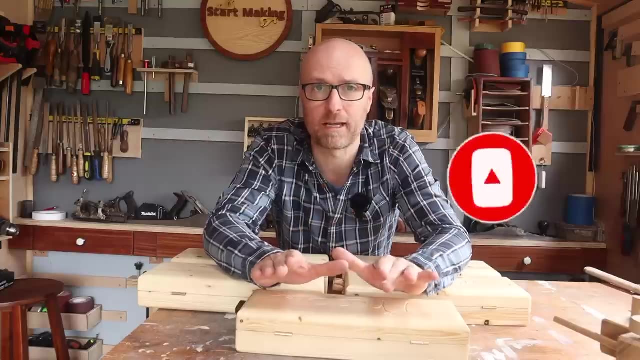 from doing a project recently. These are the upsells you can do and these are the things that make these unique. I'm going to show you some finished products up next. I favour two different ways of finishing. First one is the simplest, easiest and quickest and that is just spray lacquer, Or I go for a hard wax oil. 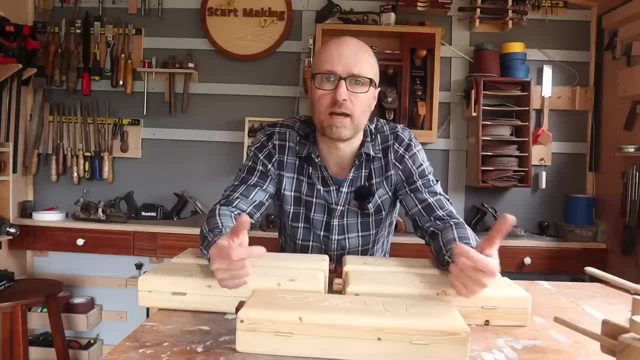 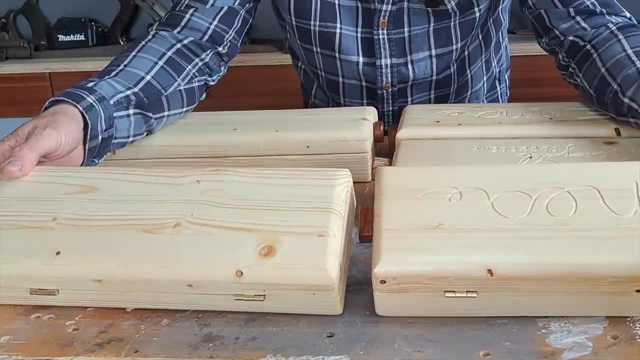 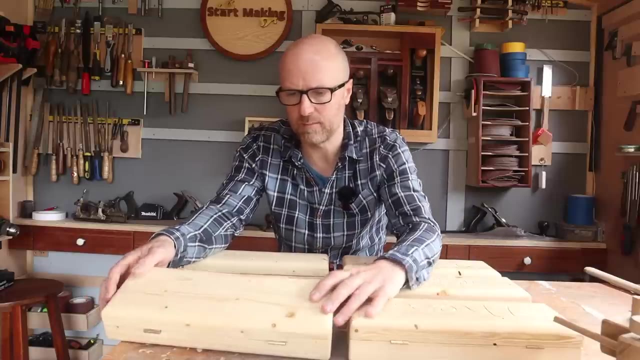 something like Osmo oil, where it takes a little bit longer because you have a longer curing time, but again it is so easy to apply. both of them tend to amber the wood a little bit, the lacquer a little bit more than the oil, and the lacquer will leave a sheen, whereas the oil tends to be. 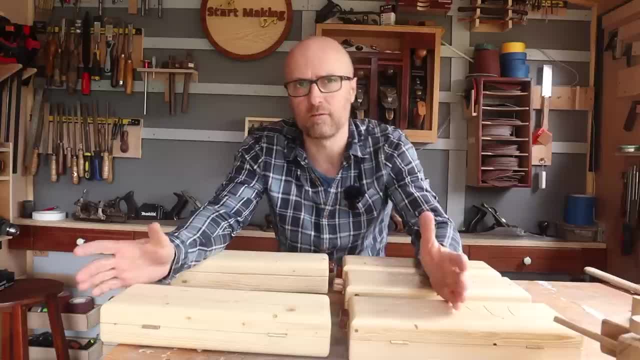 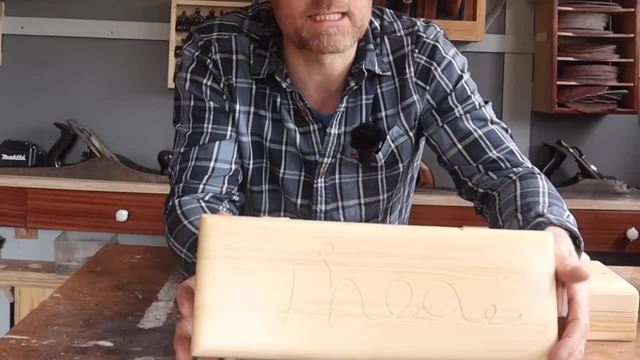 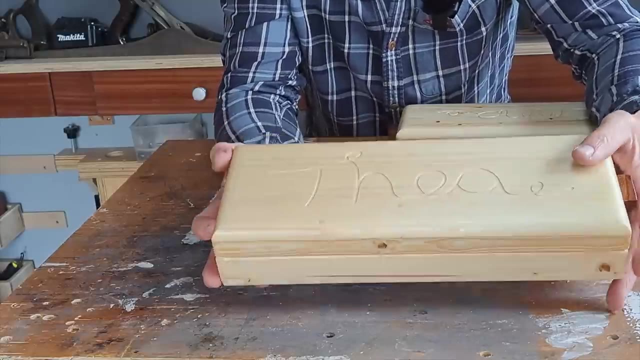 or the one i use, the osmo oil tends to be a little bit flatter. now for the fun bit. so i decided, with my router and my plunge base and limited skill and no practice, i would just write out a name and then just route it out. don't go too deep, you don't need to, and any sharp points that are left behind. 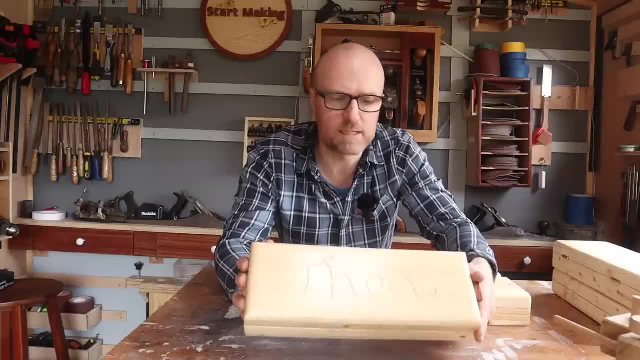 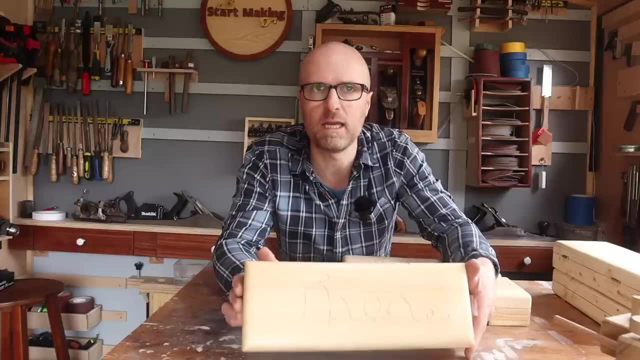 just give them a little bit of a run over with the sandpaper. whether you're offering these on facebook marketplace or etsy, have a few examples, because people can send you a name and you can route it on in. i think this took me about a minute and a half and that is an extra fiver you could. 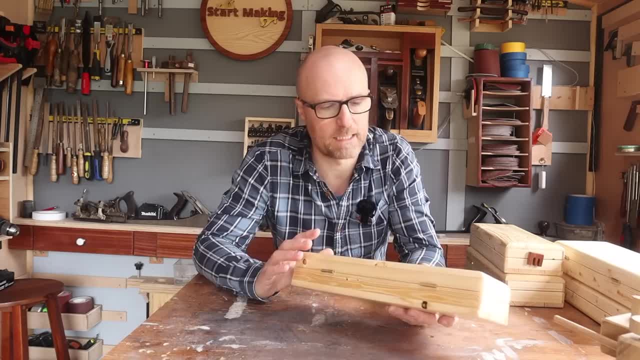 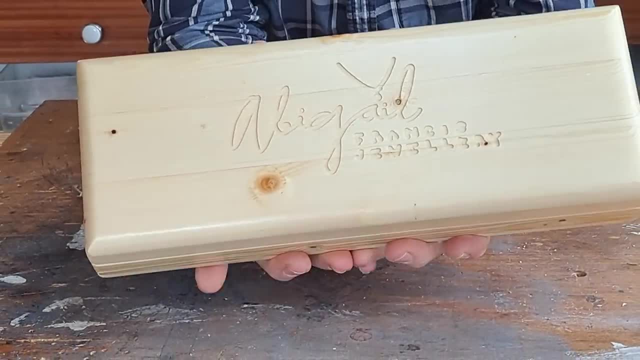 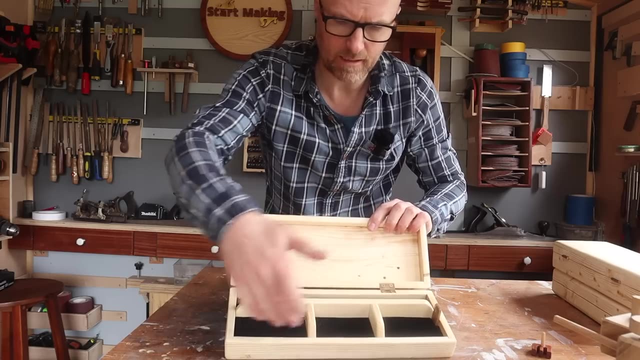 charge for it. my opinion: my wife does jewelry and i thought i wonder if i could put her logo on this, so i gave that a shot. now i will say some of the smaller letters are a little bit trickier, so so this one. i went for a long one at the back. i thought that's quite good for necklaces, and then 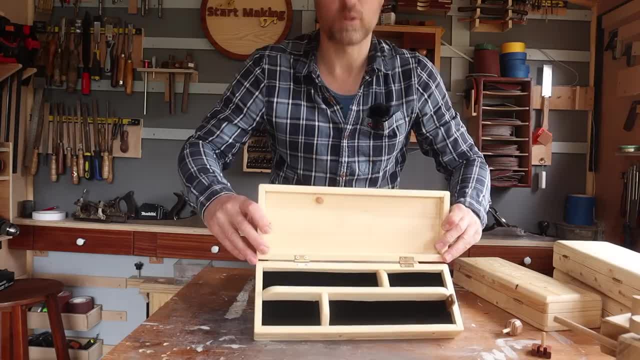 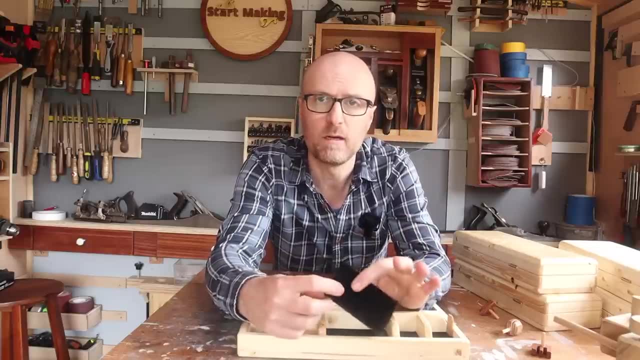 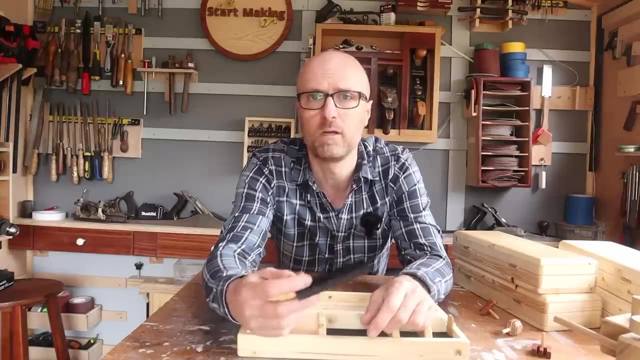 three at the front, this one, two off center and then this way this is just very cheap- amazon felt covered sponge- i'll leave a link to it in the description- and you just cut it to size with a craft knife, a scalpel, and then slide it in wedge. it i budgeted myself. 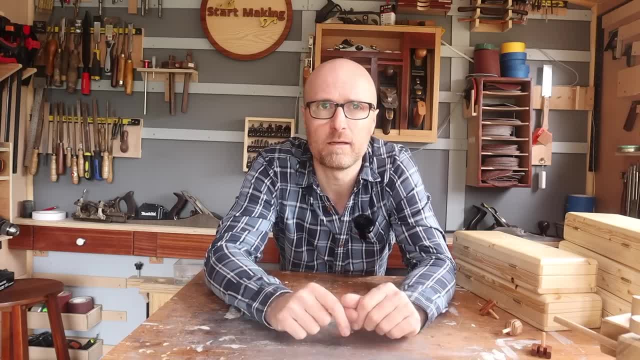 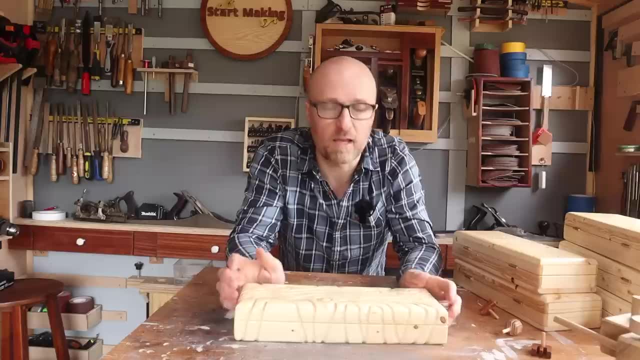 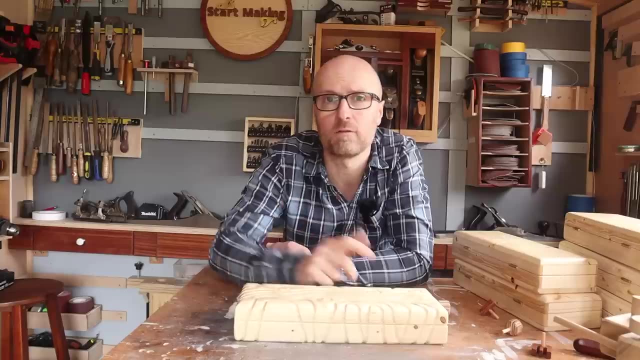 one box to do something a little bit quirky and had a lot of fun. doesn't look like much, but that was a heck of a lot of work. i think it looks really cool. i'm actually going to do a video just for this, though, because i think some of the techniques for a beginner are quite good fun. 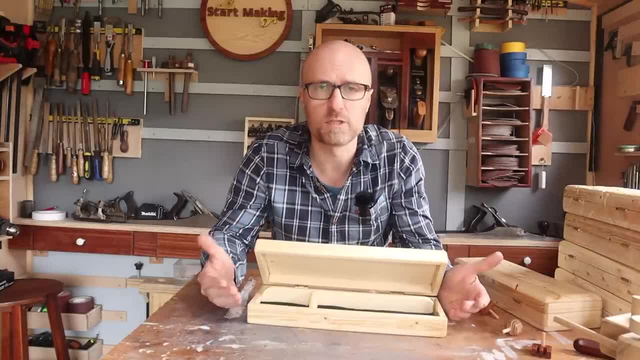 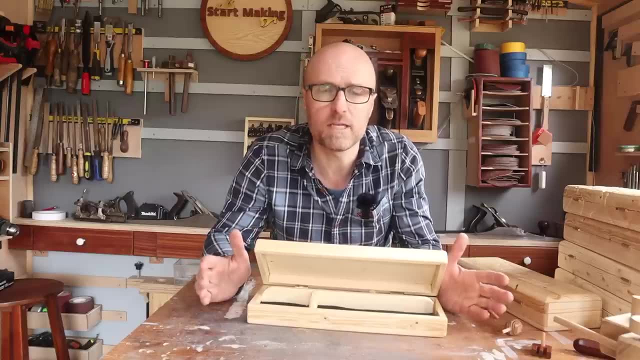 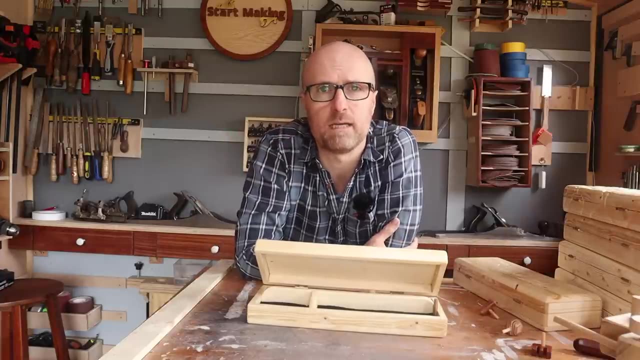 so hang fire for that if you're going to buy this wood in order to do this project. all 10 pieces of it in total came to 38 pounds. that's the entirety of the spend on wood and that's what i had left over. i spent overall about 10 pounds in hardware. take them. 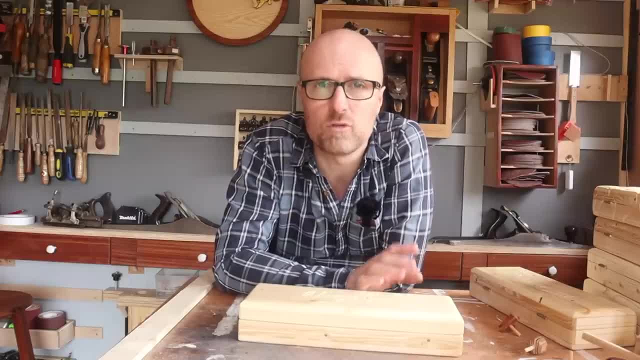 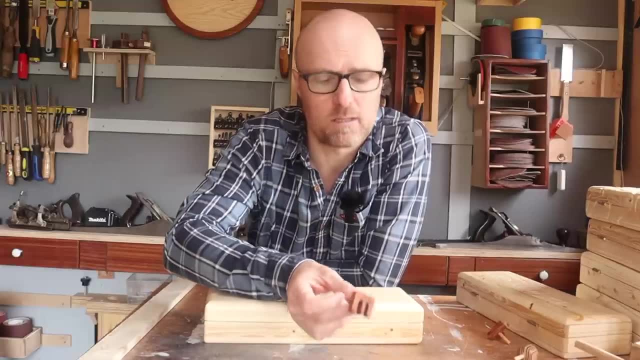 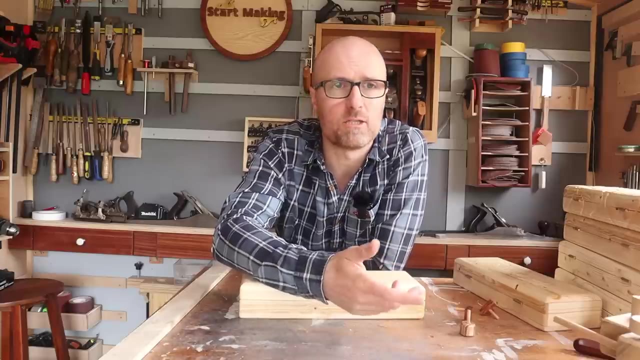 to a craft fair, stick them online, whatever amount you decide to put on them. i'm not going to suggest a price charge for the box, charge separately for the pegs. so you could do more intricate ones and try and tempt people in with a letter, or maybe just do a plain round one as your stock and then